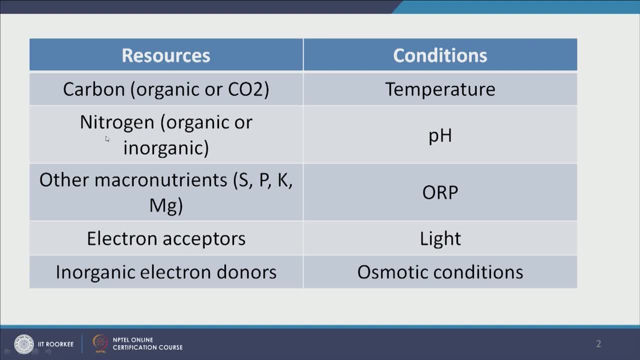 a cell. so if you remember, the DNA, the double helical structure that carries the information on how cell would live, what proteins it would make, how it would survive and its activities. so nitrogen is very essential component of the genetic material. so nitrogen should be available in its environment, either in organic form or inorganic form. now some microbes can. actually fix inorganic form of nitrogen, such as nitrogen gas, and they refer to as nitrogen fixing bacteria. others cannot, so they would require other assimilable forms of nitrogen, such as nitrate, nitrite, ammonia or organic form of nitrogen. cells also require other macro nutrients. remember the word here is macronutrients, not micro, so these are nutrients. 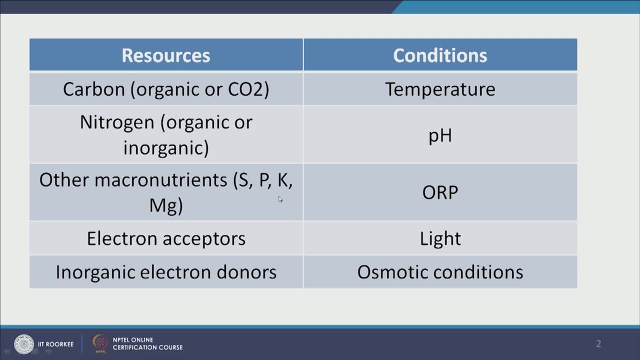 that it requires in good quantities, such as sulfur for phosphorus, potassium and magnesium, So macro nutrients. Then there are micronutrients that I have not put in this table that are also required and trace amounts. So we have talked about trace elements before, how they are essential for making certain 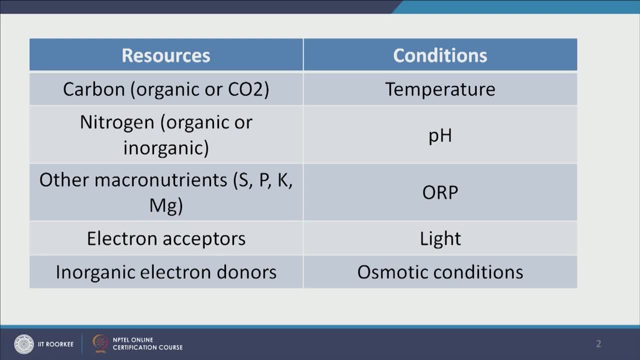 enzymes and amino acids. So we need them too, but in very little amount. Usually, microbial communities have a way of finding these micronutrients, trapping them and recycling them over and over. So the environment does not have to be rich in micronutrients, but definitely rich in. carbon nitrogen and other macronutrients. Also, the environment should have a good supply of electron acceptors and electron donors, because all life processes are a redox reaction. they are a reduction in oxidation of electron acceptors and electron donors, So it is important to have both in the environment. 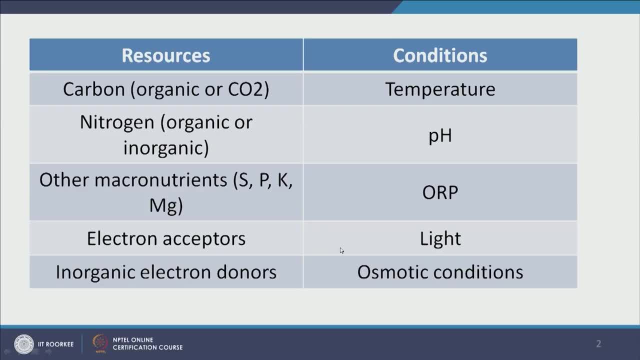 Now, when we talk of conditions, the conditions should be just right for the microbe. Now the temperature that is right for one microbe may not be correct for the other microbe. For example, if we have a thermophilic microbe. That loves hot temperatures and we put it in cold water, it will die. It has to have just the right temperature that it requires, ranging from very cold, like sacrophilic microbes, for example, found in ice sheets of Antarctica and Arctic and Himalayas, or we can have thermophilic microbes that love to be in hot water lakes or undersea. 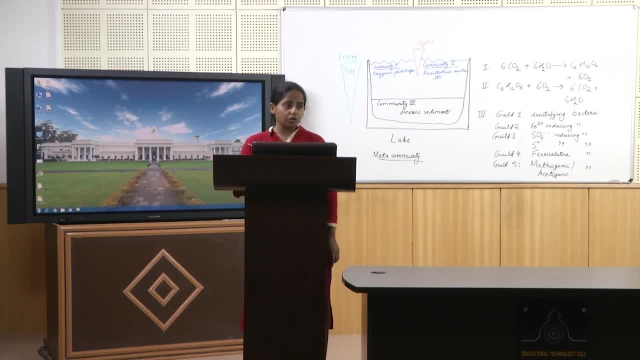 volcanic vents. Then the pH should be also right, and in one of the first lectures I talked about different range of temperature and pH in which microbes survive. So a microbe that loves hot temperatures and we put it in cold water, it will die. A microbe that grows in acidic lake will not survive in a neutral or may not survive. 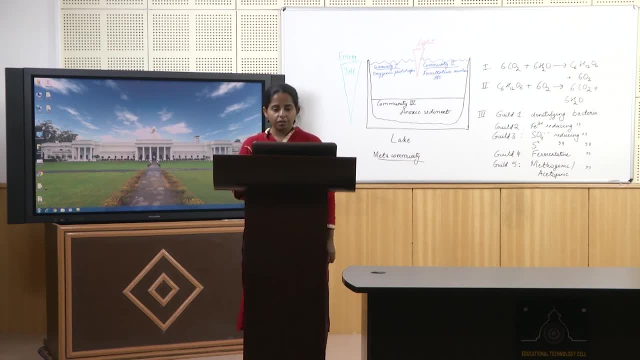 in a neutral than alkaline lake, So the pH has to be correct too. Now, thinking of temperature and pH, it is very important to note that human, not only microbe, but even higher orders of life, such as human beings, also require just the right temperature. 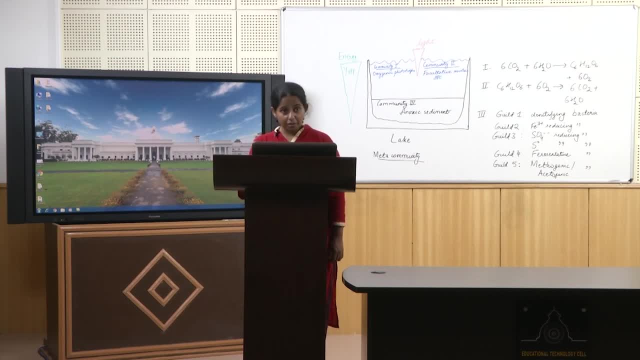 and pH. For example, life cannot survive in extremely cold environment, such as minus 120 degree Celsius, or hot environment, such as 70 degree Celsius or 80 degree Celsius, as we know it it we cannot survive, and same is true with pH If pH is very low in our environment, in 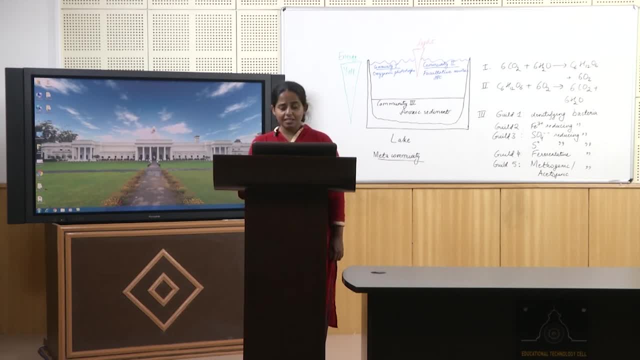 our air, we will get burned and we will die of necrosis and other diseases. Similarly, if pH is very high, we will have corrosive burns. Next is ORP, which stands for oxidation reduction potential. So basically, a methanogen which requires a very reduced environment to survive will not survive in oxidized environment. such as air. So not only does methane methanogen a methane producing bacteria, it not require oxygen, but if it is exposed to oxygen it will die. So in this case we require just the right amount of ORP oxidation reduction potential of environment. the light should. 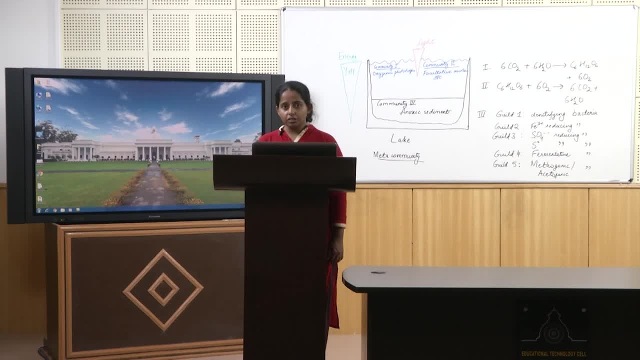 be correct too. If there are phototrophic bacteria and they are not getting oxygen, they will die. and the osmotic conditions? If you remember, we have talked in one of the early lectures that cellular membrane is a bilipid in bacteria. 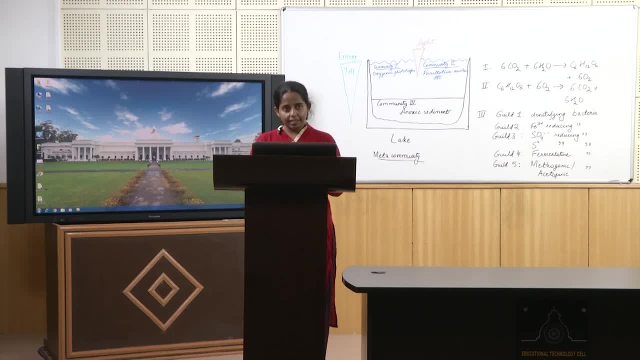 And it has hydrophilic and hydrophobic end. So inside the cell there are there is some osmotic pressure relative to outside of the cell and if there is change in external conditions, the osmotic pressure in external condition, the cell might either explode or implode. For example, if I take microbes that live in hypersaline environment, like ocean, and then put it in a fresh water bowl or fresh water lake, then they are likely to they likely to lose their integrity. Same is true otherwise, if we take water from, if we take microbe from. 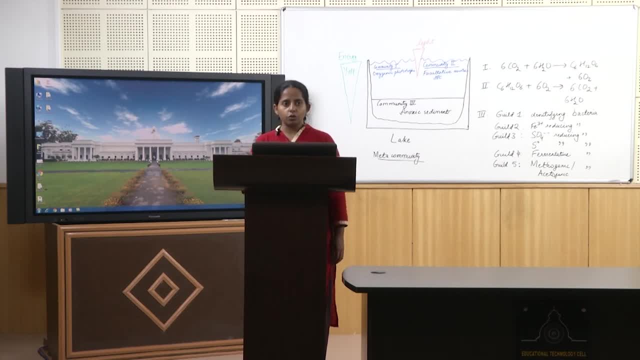 a fresh water lake and put it into a saline environment, it will also lose its integrity and not survive, most probably. Then, another thing we need to understand, So this is microbe in a individual level. we know what microbes require on individual level: what resources, what conditions. Now let us look at what microbes require when they we 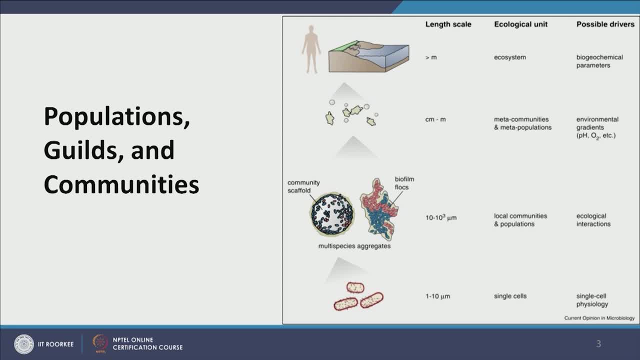 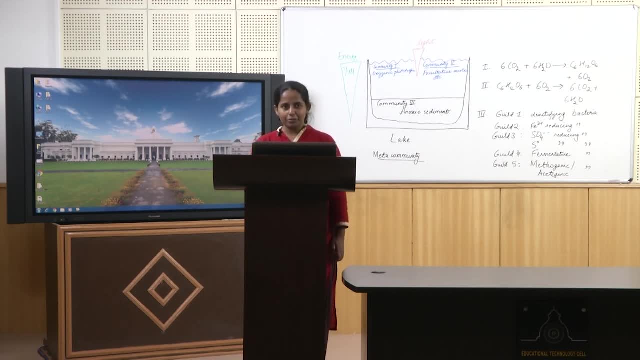 are talking about many microbes present together in an environment, because there is hardly any environment where there is just one microbe sitting and you are looking at just one microbes need. Usually it is either a population, guild or community. So now is a good time to introduce 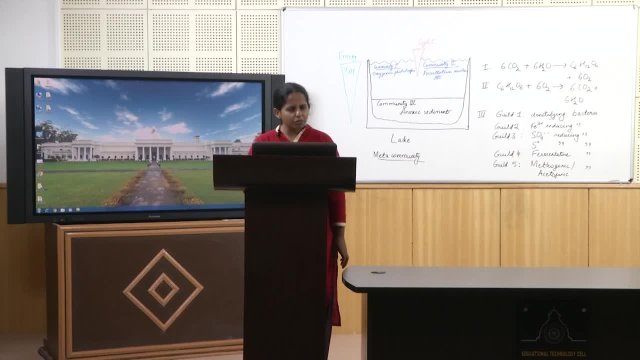 you to the concept of population, guild and community. I have sort of mentioned this before, but let me be very clear. Population is when many microbes belonging to same species are together, So we might have population of equal life. they all belong to same species. 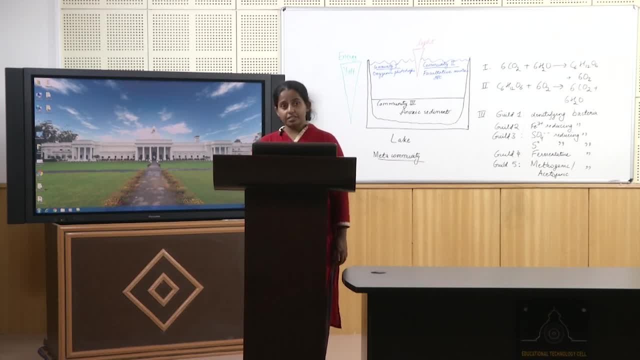 On the other hand, community is when different population. So we might have Ecoli, we might have Pseudomonas aeruginosa, we might have some other. 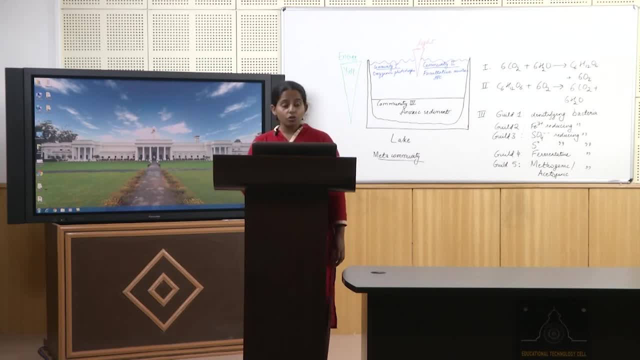 microbe acidobacterium coming there. So we have multiple populations, so we have lot of microbes from different species together. they are interacting with each other. yeah, this is community, microbial community. And now the third word is guild. now, guild is a group of microbes that are same in their 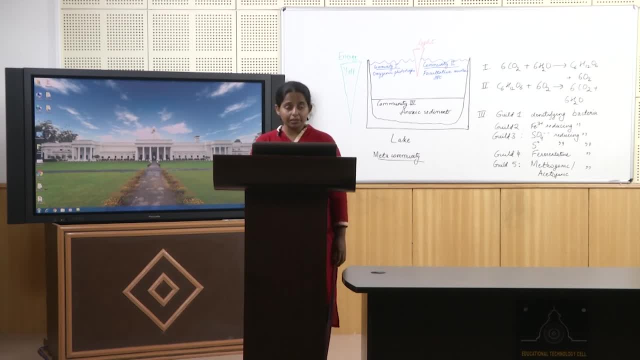 function- and this I have talked a lot about when I was talking about metabolism of microbes in previous lectures- that because the ORP, or oxidation reduction potential of an environment is bound to influence all the microbes that are present in the community, they are likely to have similar functional traits. 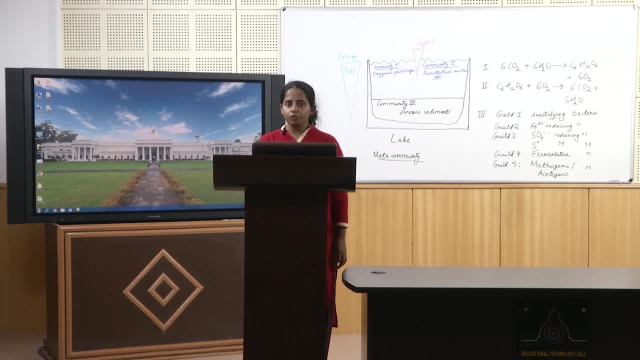 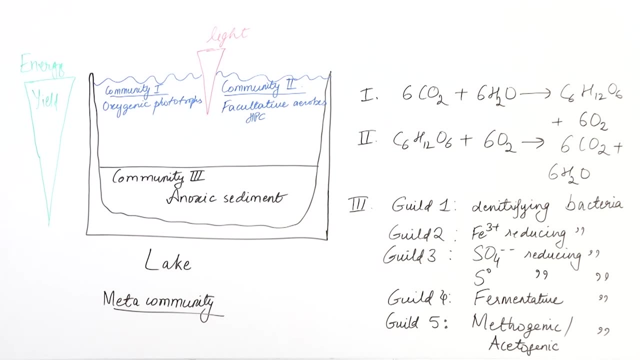 And we will go about this and I will show you right away what we mean when we talk about guilds. So, students, now let us take a look at population, guilds and communities within one particular environment. Here we have a diagram of lake, a very rough schematic, and what is in blue and wavy is 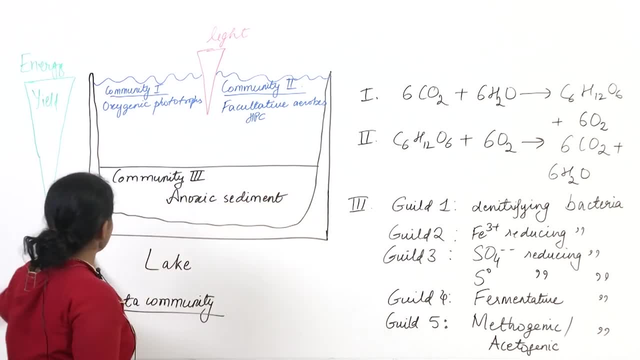 water and this is the sediment, and this is the control volume boundary that I have drawn for the lake, and this is a cross section, by the way of the lake. So let us look at the microbial community present in the lake. So where look? here the red arrow is showing you the depth until which light can penetrate. 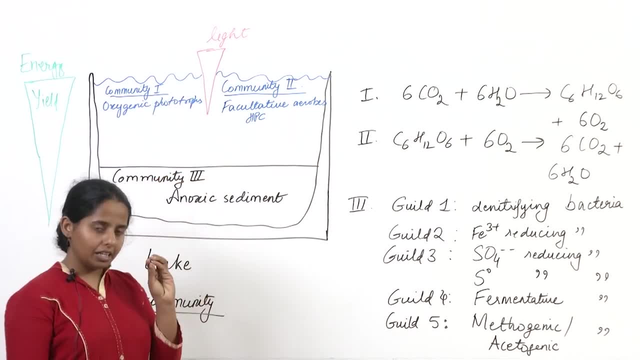 and its width can penetrate. So this gives you an idea of the intensity of light that enters and reaches at this particular depth. So until where the light can reach, we can have two kinds of microbes, where in the first microbial community we have oxygenic phototrophs. 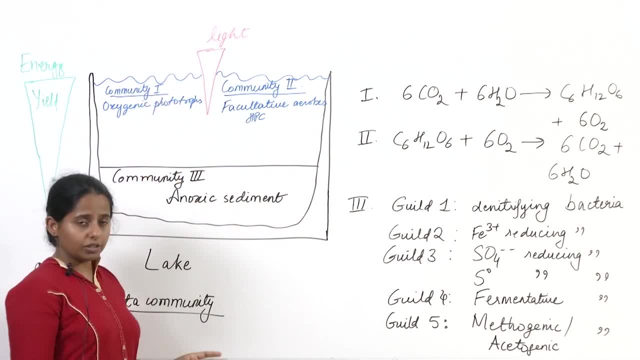 So remember, because this is towards the surface of the lake, we will have reaeration and aeration going on, and thus oxygen will also be present in the top surface. So microbes that can utilize the light produce food by consuming carbon dioxide as the source of carbon. they will be present here. 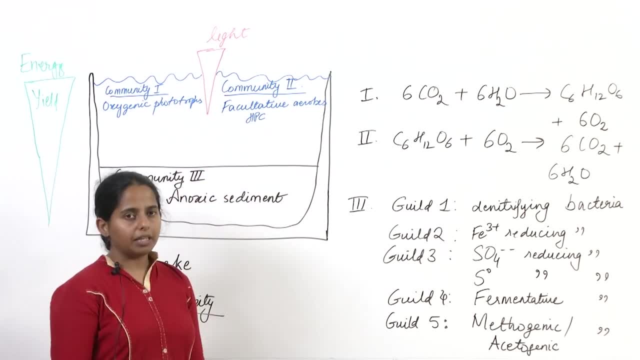 The other kind of microbes that will have here will be facultative or obligate aerobes that require oxygen. as I mentioned, oxygen will be present here. So the first kind of microbial community. now, remember I am calling this microbial community So it implies that there is not just one oxygenic phototroph but there are multiple. 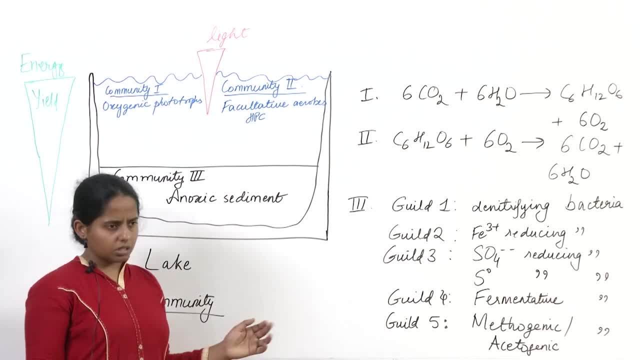 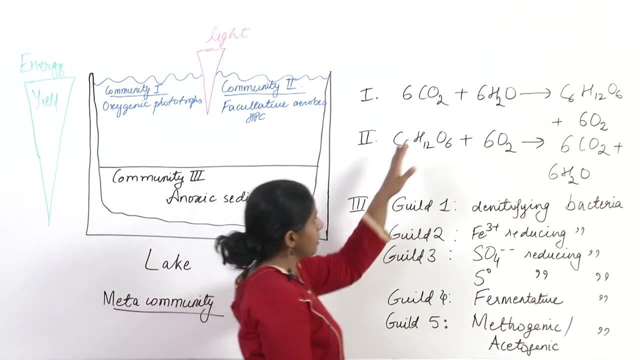 species of oxygenic phototroph that might be present or in certain unique environments. you might only have one single population of oxygenic phototroph, or facultative aerob or obligate aerob. Now, in community 1, the one that is a phototroph. they use light, they use carbon dioxide and 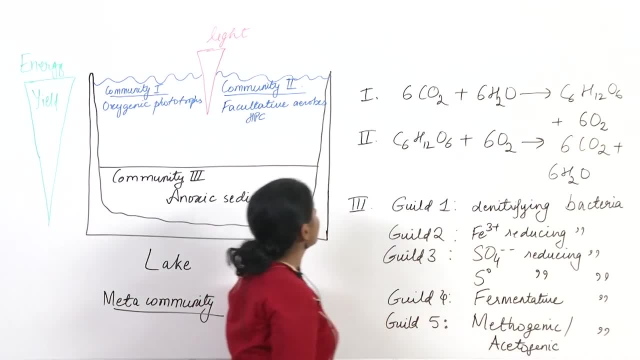 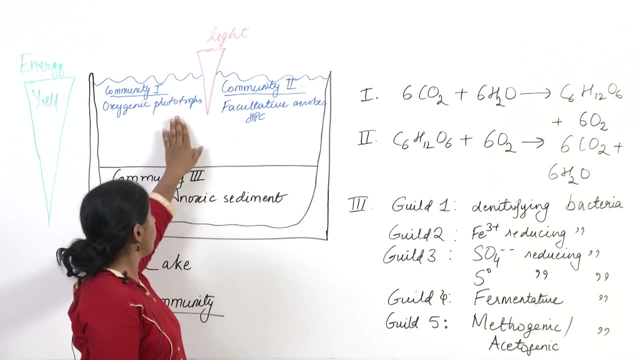 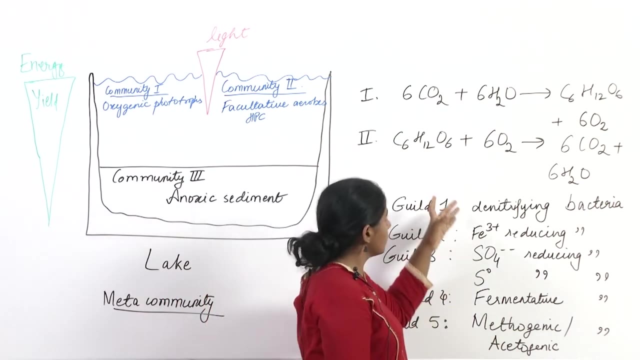 water and produce glucose and oxygen. Now facultative aerob are in cooperation with them. they are very happy to live next to the oxygenic phototroph because they are producing oxygen and they are producing glucose. Facultative aerob, and aerob in general, can consume the glucose by using oxygen as electron. 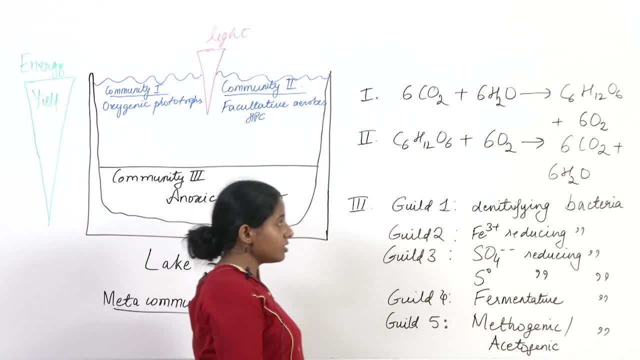 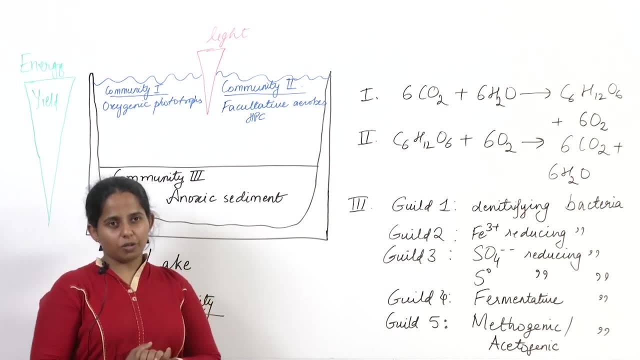 acceptor and get tremendous amount of energy from here. So this is- and produce carbon dioxide which can be consumed by oxygenic phototroph. So this is an example of cooperation between two different microbial communities. Now, in towards the sediment or towards the bottom of the lake, we have anoxic zones and 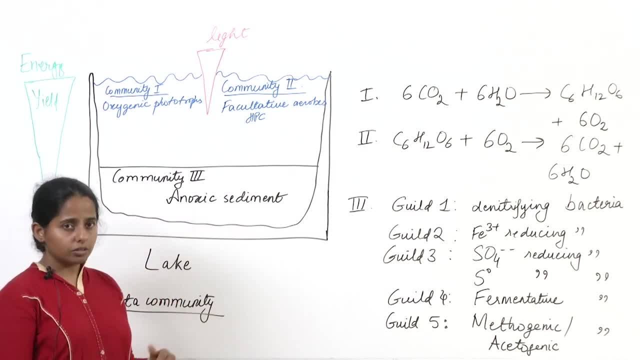 we might even have completely anaerobic zone. So anoxic zone has, like, trace amount of oxygen present, So in sediment for example. we might have third kind of community, that is, lives in anoxic or anaerobic environment. Now, in this particular community we might have at the top layer, let us say there is 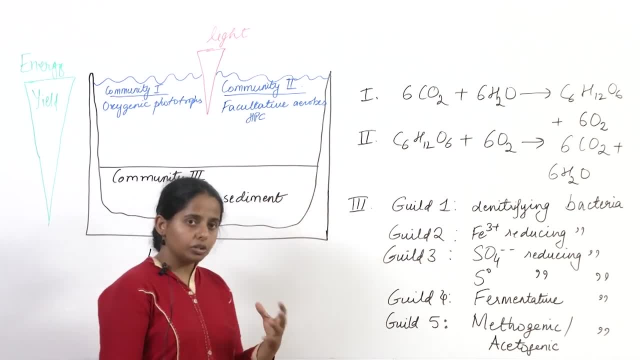 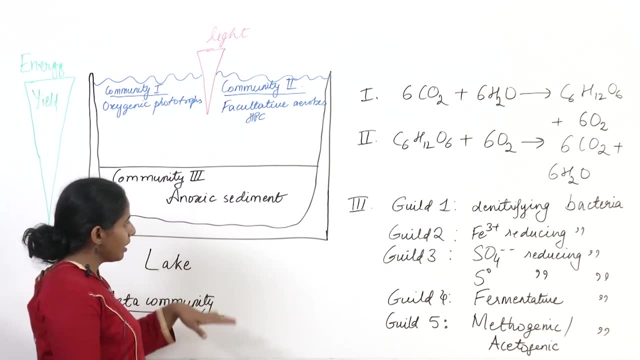 some amount of nitrate present Now, so the microbes that can utilize the nitrate. why did I say top layer? because, let us say, initially, when the lake was built- let us say it is a manmade lake- there was nitrate present here, So microbes started utilizing nitrate. 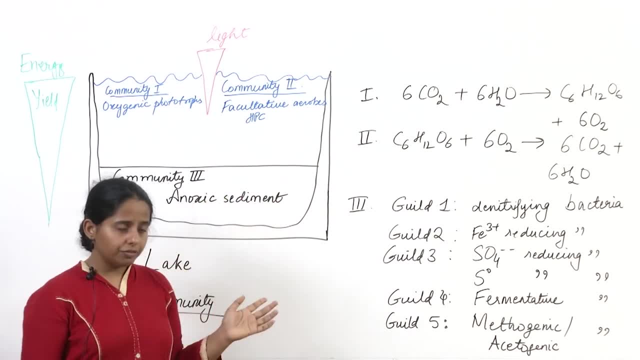 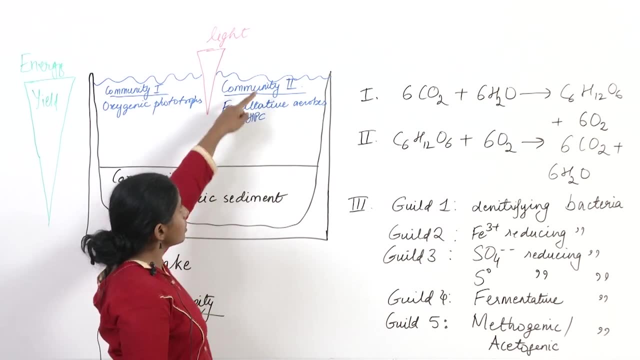 And as the nitrate depleted, they moved on to different electron acceptors and they made a gradient of electron acceptors over time. Why would they be a gradient? because, remember, the oxygen is coming in from here and oxygen as it comes in, if nitrate has been denitrified, it will oxidize it again. 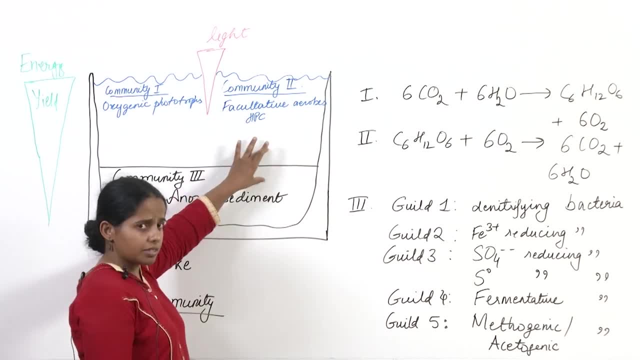 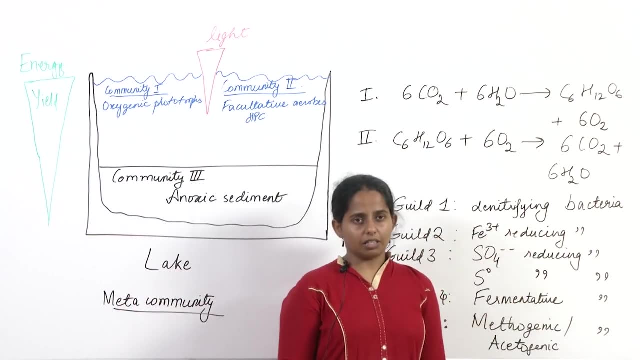 So there is higher chances of nitrate to be present on the top of this sediment layer than on the bottom. So one guild or one functional community of microbes could be denitrifying bacteria, So bacteria can be oxidized. So bacteria can be oxidized. So bacteria or microbes that denitrify. they are one functional group and they are likely to be found in the top layer. Next we have the second guild, which is ferric reducing bacteria. So when, let us say, nitrate got depleted and now we have ferric ions present. 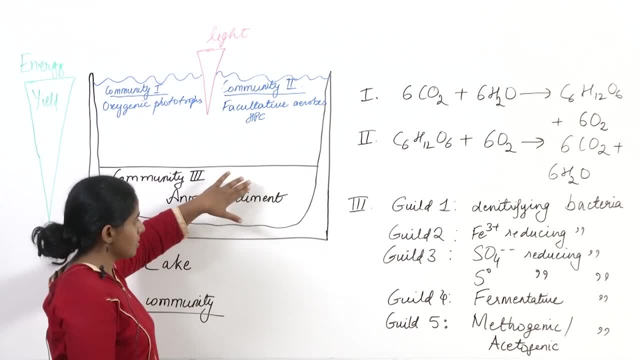 So microbes that can utilize that, reduce them and get energy, will be present here. The third guild, and most probably below it, would be sulphate reducing bacteria, followed by sulphur reducing bacteria, and then fermentative microbes, And then methanogenic and aceticogenic microbes. 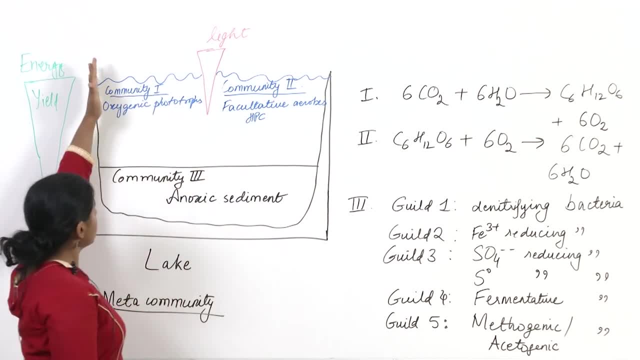 So you notice here that as the electron acceptor gradient, So as we notice here that the microbial community gradient follows the electron acceptor gradient. So here we have oxygen, then we have nitrate, we have ferric, sulphate, sulphur, Then we have fermentation condition and then methanogenic and acetogenic conditions. 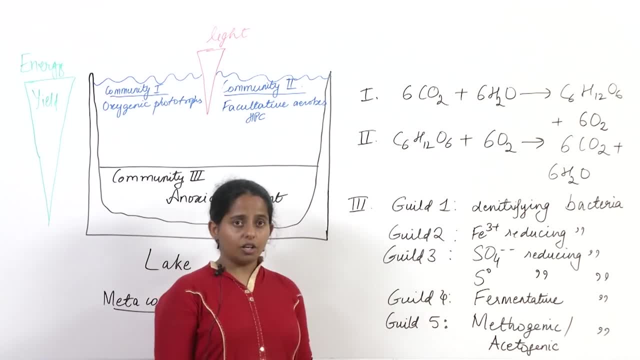 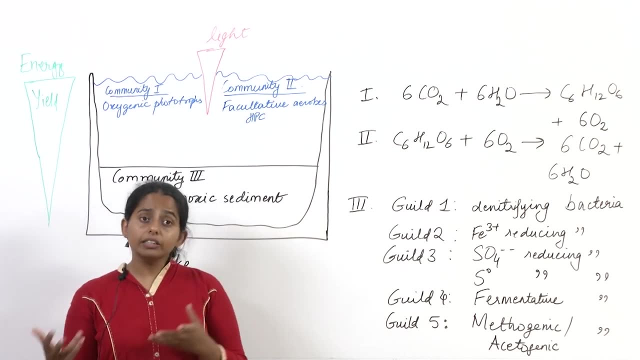 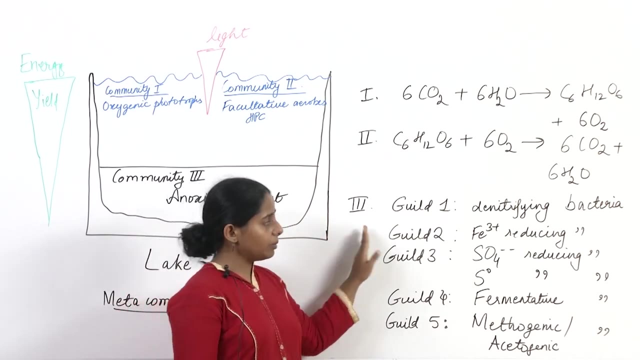 So a guild are microbes that have same function are iron reducing microbes. they form one guild, all microbes that are iron oxidizing microbes. there are other guild now they might have different populations within them. So within guild 2 there might be many different kinds of iron reducing bacteria within. 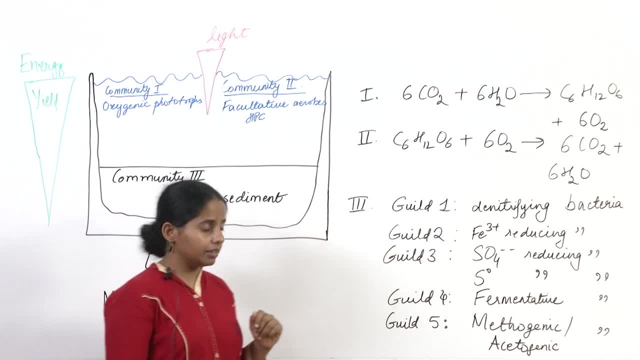 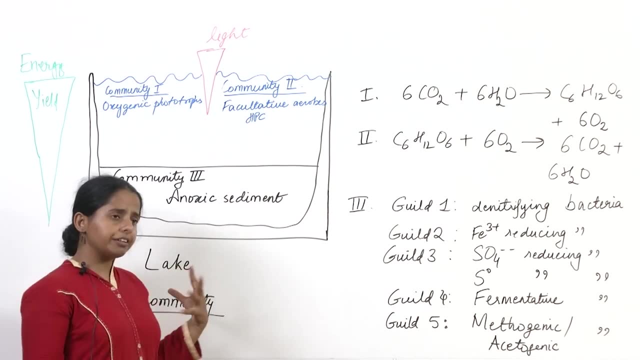 sulphate reducing bacteria. there might be very different kinds of sulphate reducing bacteria, So a guild might have singular population or it might have a community, but the unifying factor for a guild is that their functional characteristics are same. Now, as I mentioned before, population, you should remember, is one species only. over all this, 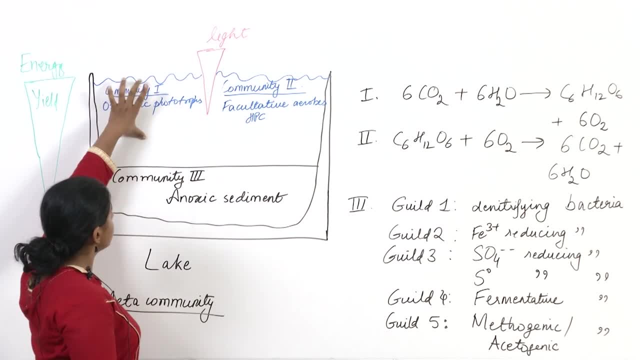 together, So a community would be here. you know, the environment is similar, right, their functions are sort of similar: multiple populations living and interacting with each other. So this is one community, community 2, community 3: within each community there are multiple. 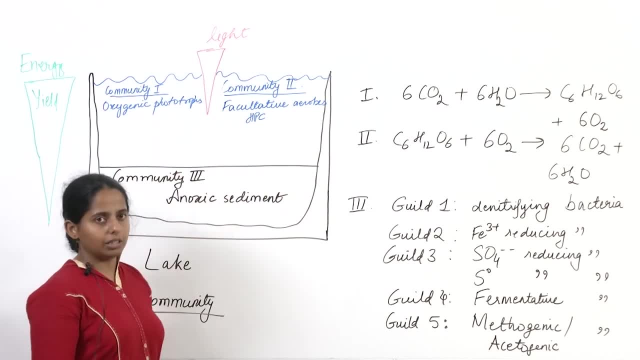 populations. together they make a meta community clear Now note here. So, from top to bottom, we have a gradient of oxidation potential, oxidation reduction potential. we have a gradient of electron acceptor, therefore, and we also have a gradient of the kind of microbial communities we will have. 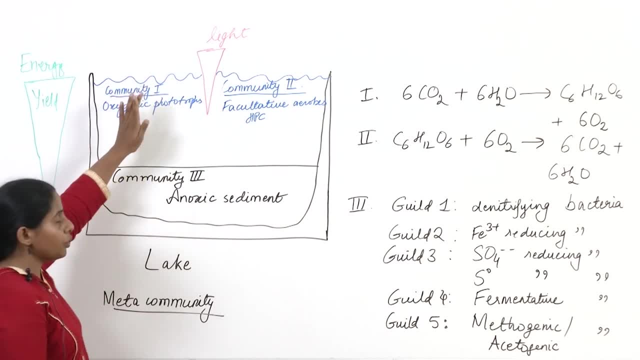 Now, because oxygen is energetically most advantageous. we also have a gradient of energy yield, So the microbes growing on the top of this lake would have, would get the highest energy yield And the ones on the bottom that are methanogenic or acetylene. 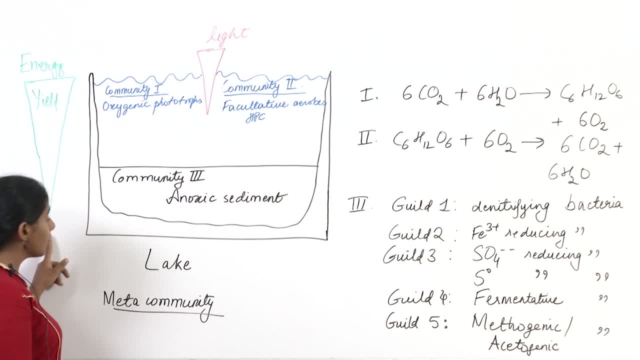 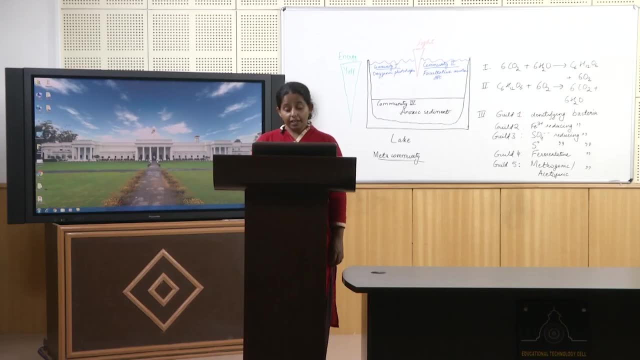 So the microbes growing on the top of this lake would have would get the highest energy yield, And the ones on the bottom that are acetylene or acetogenic will have minimum energy yield. alright, So to revise, we have single cell physiology. 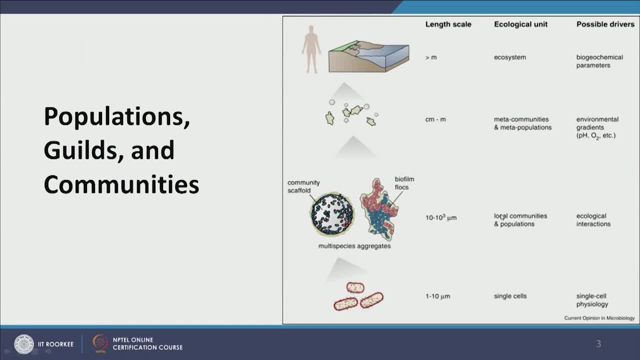 So we have single cells and then we have local communities and population. remember, population is microbe of same species. communities are different populations existing together. For example, in this microbial flock we have microbes stained red and microbes stained blue. all together, this is a community. 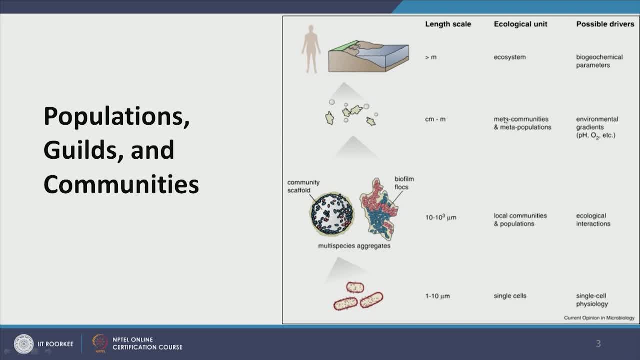 So we have single communities and metapopulation, So a metacommunity and a metapopulation- the example would be the lake that we just saw- and then we have ecosystem, So we have the entire region that includes aquatic components, terrestrial components. 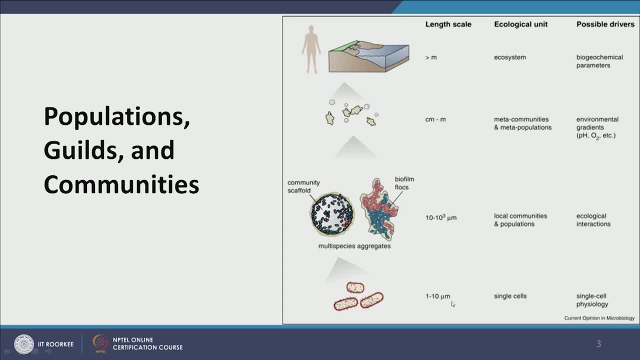 and air components. So the range in size also varies. our single cell can be anywhere from 1 to 10 micrometer. the communities and population can be anywhere up to 1000 micrometer. the metacommunities, metapopulation, and we will see some of them today in lecture. 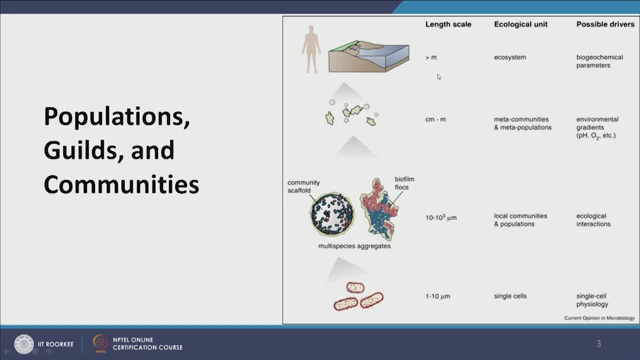 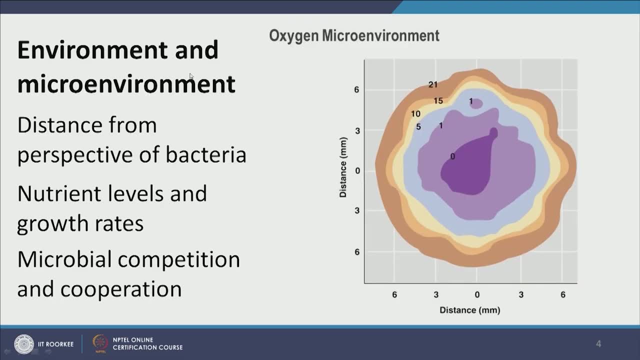 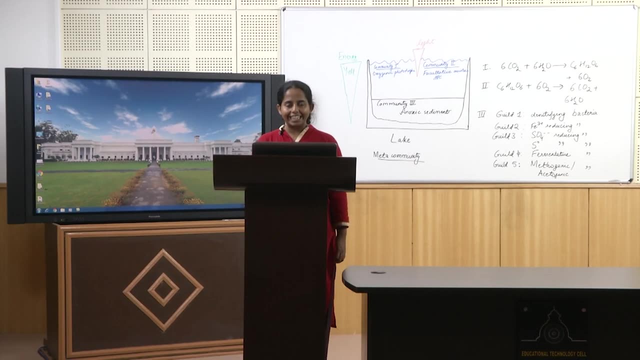 Can be up to meter and ecosystem more than meters, many meters. So now let us look at environment and microenvironment of microbes, their populations and their communities. So when we talk of environment and microenvironment, let us try to get in perspective of bacteria. 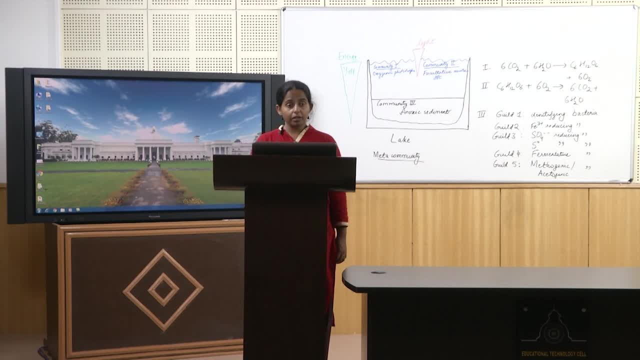 or a microbe on distance. So for a human being a 10 centimeter is not a long distance. So 10 centimeter we can just approach it very easily. But now think from the perspective of a microbe that is only few micrometer in length. for 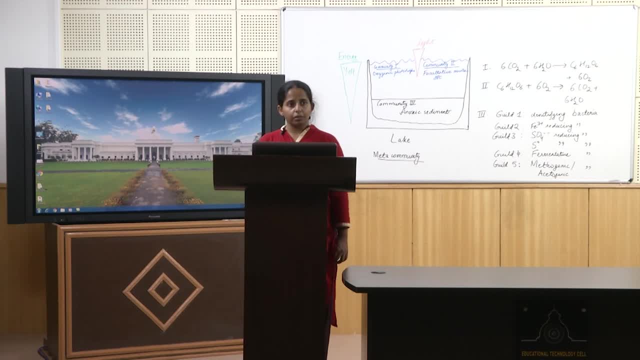 that microbe 3 millimeter can be as long as it is as 2 kilometers is for human being. So within 2 kilometer ADI, we can have different, as we know, we have different populations of higher order of life. we can have monkeys, dogs, cats and rats, and human beings again. 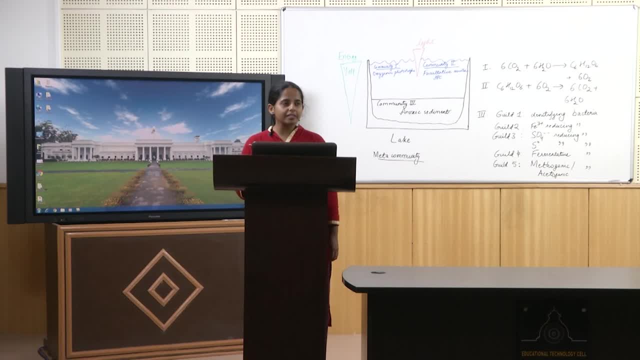 human beings all following different practices here, different food habits. Similarly in for microbes within 3 millimeter space. it is a very small space from human perspective but it is plenty from bacterial perspective that we can have microbes, bacteria of very different functions, of very different populations. 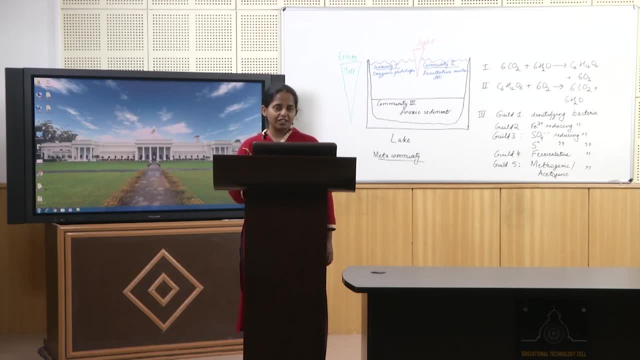 So within 3 millimeter space, we can have very, very diverse community as diverse community and even more diverse community than we have when we talk about higher order of life, like birds and animals and humans. The other thing is within 3 millimeter radius. you might say, well, it is just 3 millimeter. 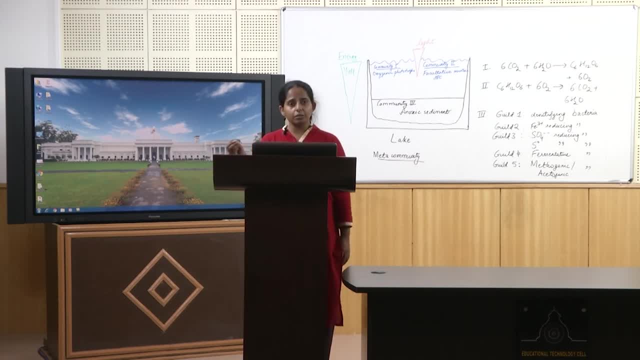 the environment would not change a lot. So the microbes within 3 millimeter should not be very diverse. but the beauty here is that in the micro scale we notice that environment changes. the gradient of rate of change of environment is very high. Now on the right panel here I have a picture. 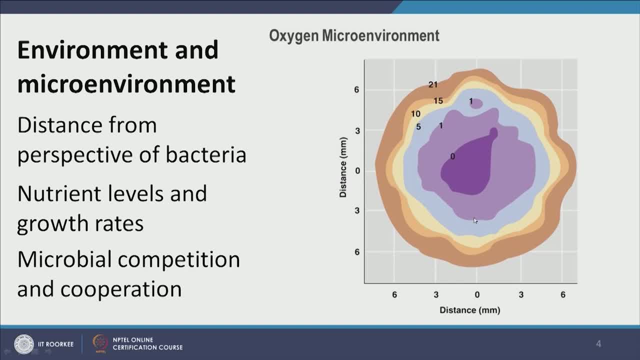 And this is a cartoon, a schematic, showing you the oxygen levels in a soil micro pore. So you know, soil has pores, where through which the air and water are transported. Now, this is a micro pore, So even among pores it is really small and we notice that this is some 12 millimeter. 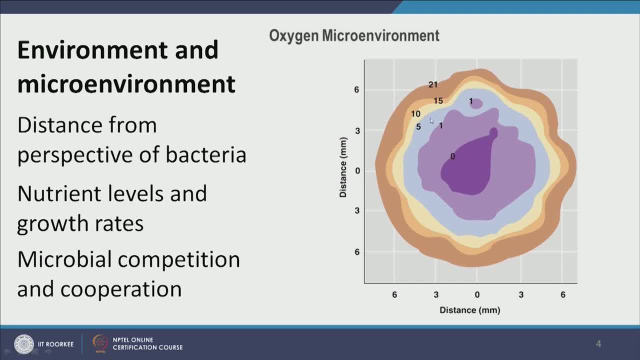 in diameter and now what you are seeing in different colors is oxygen gradient. So in the brown you have the highest amount of oxygen and it reduces that. it goes to orange and then lighter yellow and then blue. Then you have the red, A little bit light purple and then dark purple. there is no oxygen left. 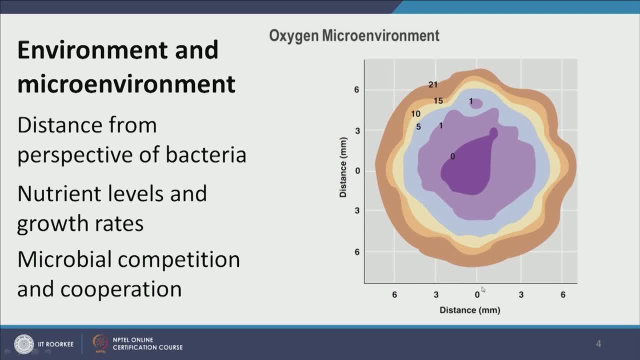 So within this 6 into 6 millis- So we have 12 millimeter range- we can go from aerobic microbes to fermentative, methanogenic and acetogenic bacteria. So think about it this way and it is. if you look at, even this is too big of a micro pore. 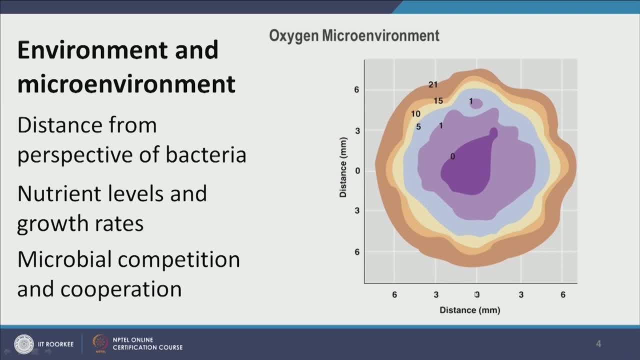 by the way, even in pores as small as 3 millimeter we have seen similar characteristics, similar behavior. So in the dark purple region we might have methanogens, acetogens, we might have sulfur reduction, sulfate reduction, nitrate reduction, nitrate reduction and then obviously, oxygen. 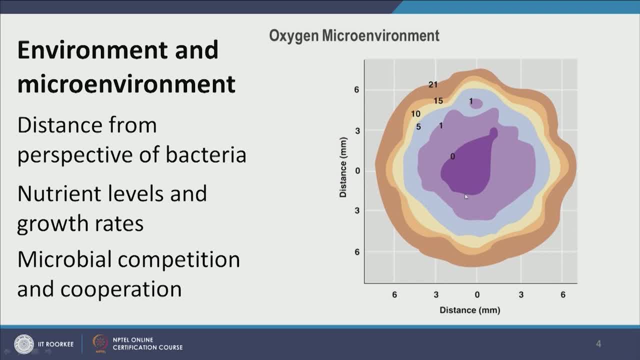 reduction. Now, now, all this diversity in the ORP oxidation reduction potential of this micro environment will result into diverse functional diversity of microbes which will allow a community, very diverse community, to grow in this 12 millimeter by 12 millimeter micro environment. 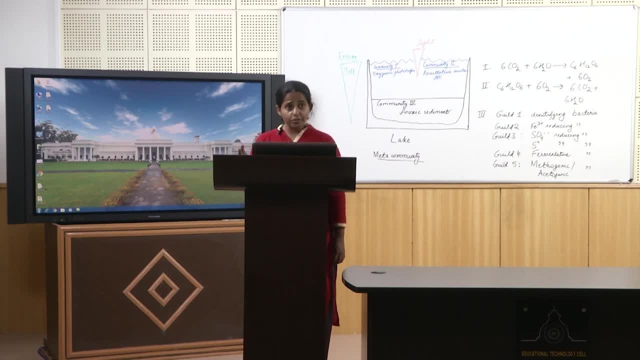 Thank you. Now, all these microbes of different kinds. they will compete for resources. For example, in the aerobic region denoted here by dark brown, we not only have one singular kind of aerobic bacteria, or archaea, or eukaryote, but we have different kinds of microbes and 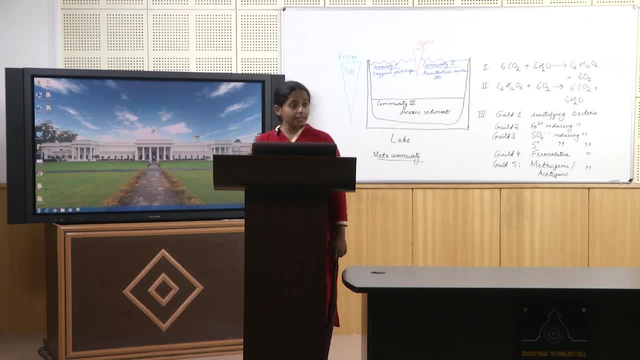 all of them are competing for oxygen. So the one that can grasp oxygen fastest, the one that can degrade its electron donor fastest and grow fastest is likely to outcompete other microbes. Thank you. But then there are other factors also that influence microbial growth: microbial competition. 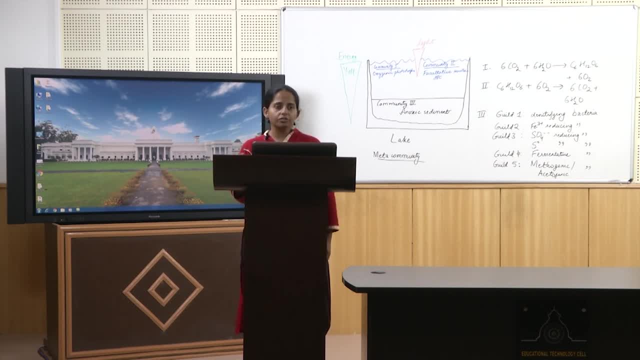 So now about microbial competition. because of this we notice that over time the microbial communities undergo succession. So initially we might have 10 different aerobic microbes here and after some time we notice we have 8 because 2 have been wiped out. And let us say microbe population number 4 was the most abundant initially, but now that 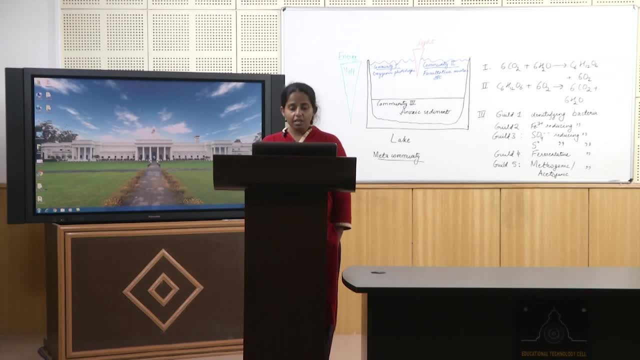 might have been outcompeted by 10.. Thank you, And let us say microbial population, number 6.. So we notice that microbial communities undergo succession over time because of competition, And on the other end of the spectrum we have cooperation, So microbes cooperate with each other. 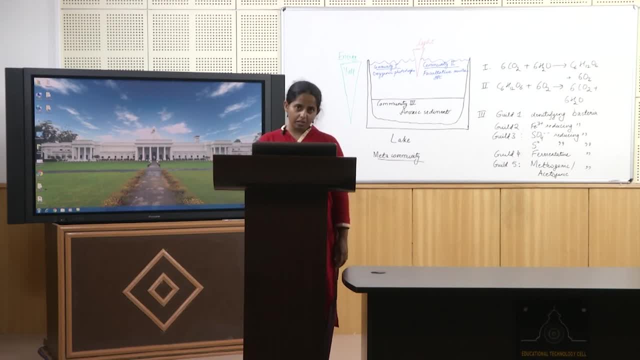 For example, someone's waste product could be someone's input, And in next few slides we will see how microbes not only cooperate with each other, but they also cooperate with higher order of life, such as plants and such as humans. So we remember this is one of the first things I talked about in introductory lectures. 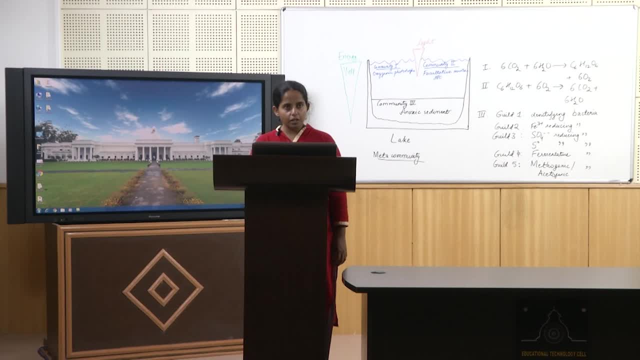 that we have more non-human cells in our body than we have human cells, begging the question how human we are. So, for example, in our gut, we require certain microbes to give us a healthy functioning of gut, And when that microbial balance gets upset we have diseases such as diarrhea and irritable. 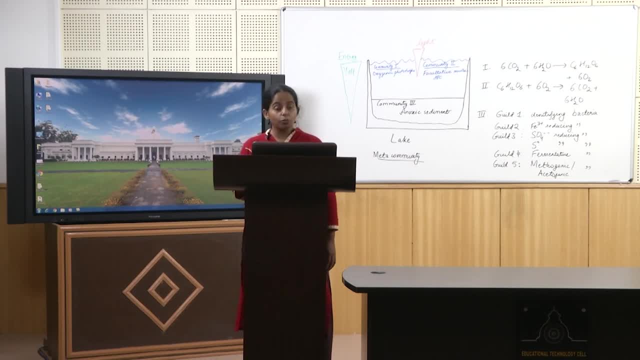 bowel syndrome. So microbes are very important in terms of both competition And, by the way, this diagram should remind you of what we just studied in the lake, how different kinds of functions, functional gradient, can be found in an environment. So now let us look at surface in biofilms. 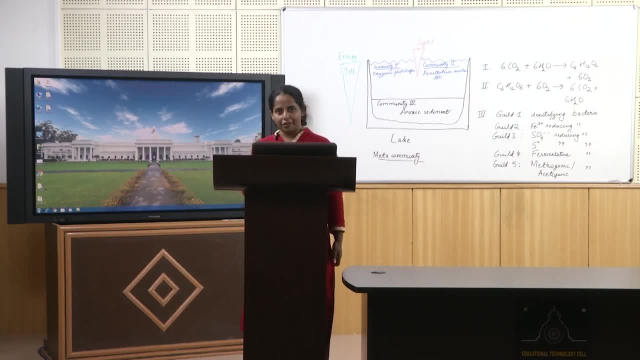 Until now, we have not talked about how microbes interact with the environment. We know they are there. are they just sitting there? are they attached to where they are sitting, or are they floating in water? Yeah, Or flying in the air? So let us start with understanding how microbes interact with surface. 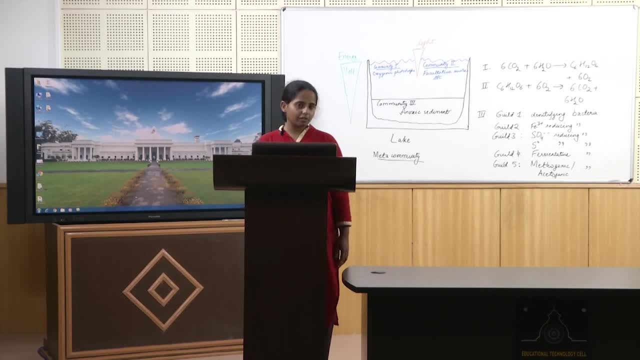 We know that many microbes love to attach to a surface and there are many advantages why they would love to attach to a surface. For example, let us say we have a stream with relatively low amount of organic material, low amount of electron donors and electron acceptor. it has good electron acceptor: oxygen. 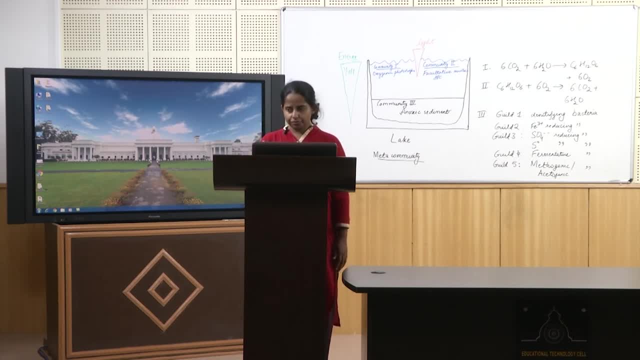 So it is a very healthy stream and it is flowing down Now as it flows down. As it flows down, it interacts with rocks and other surfaces where microbes can attach. So the microbes in water itself do not have lot of food to eat, but once a microbe attaches, to the rock. it now has a perspective from which it can stay stationary and capture all the nutrients from the flowing water. So attachment has an additional advantage that microbe can capture nutrients in flowing water. So microbe is flowing with in an oligotrophic environment, which means in a nutrient deficient. 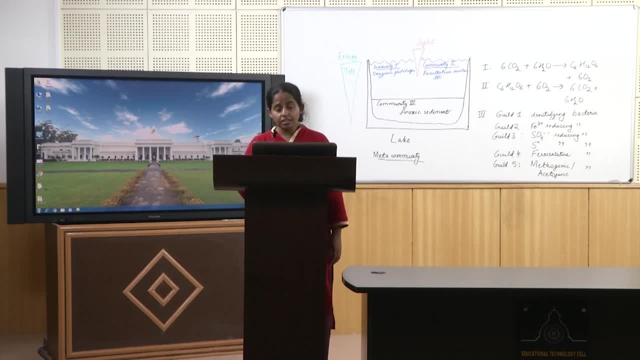 environment. So it is advantages for microbes to attach. There is another reason why microbes would love to attach to a surface. When they attach to a surface and they replicate, they produce daughter cells and the daughter cells also attach to replicate over time. what we might have is accumulation of material. 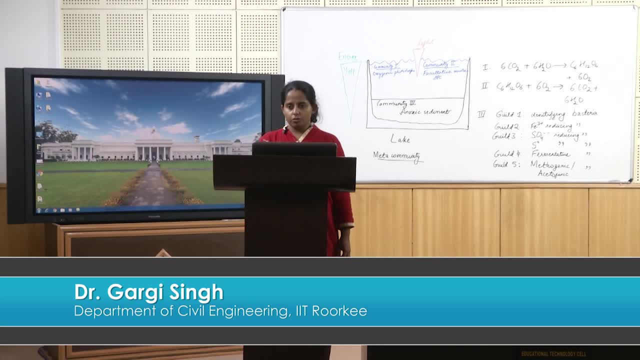 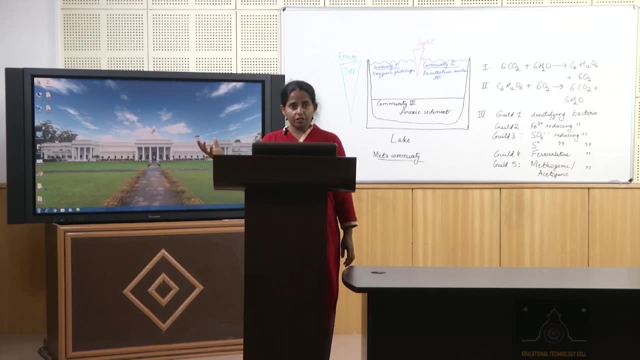 So initially we have just a plain surface with one water. So we have a surface, So we have a surface, So we have a surface, So we have a microbe attached. Microbe replicates produces two daughter cells and so on and so forth. replication continues. 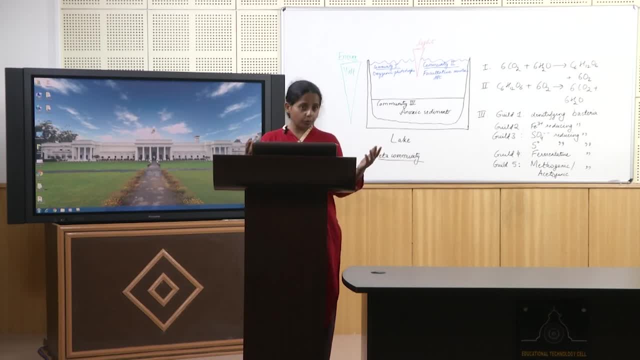 Over time we have a heap of microbes. Now we are talking about a singular population, but then we can also have communities, complex communities of microbes. Now, if microbes are faced with some problem like a disinfectant, then only the once, only. 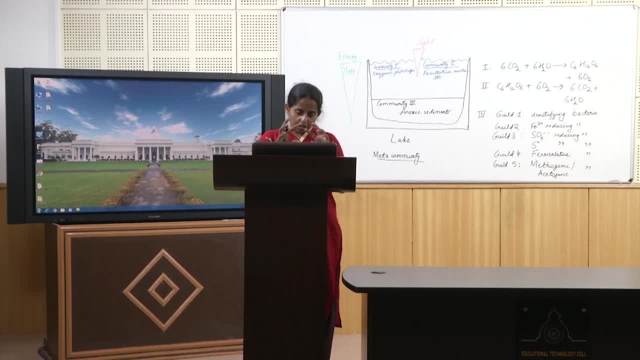 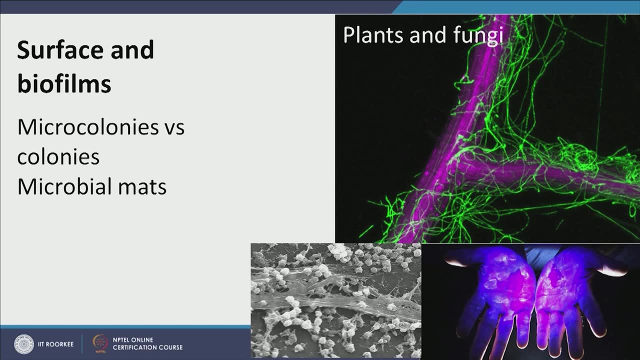 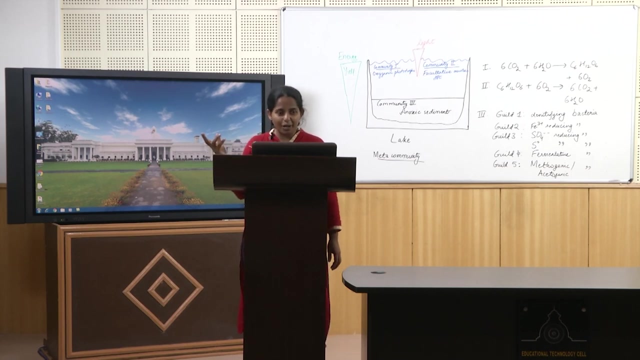 the microbes on the boundary would be affected and the microbes closer in this accumulation, this heap of microbes will be not various Effected surface attachment and growing this films on a surface actually ensures longevity of microbes. The other advantage of attaching to a surface and growing these films they refer to as biofilms. 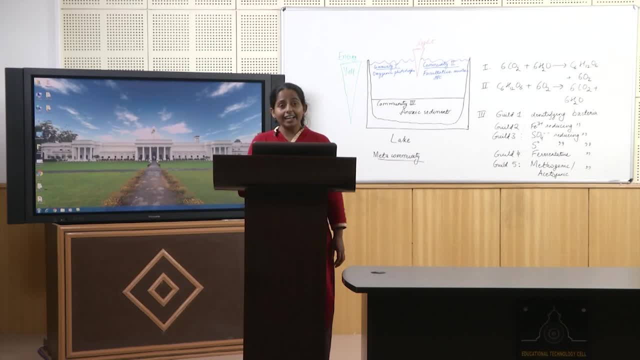 by the way. So we have here the second term, biofilm, is that these biofilms, microbes and biofilms. they secrete what is called as EPS, So these are extracellular polymeric substances that create a mesh in which the cells can trap not only themselves but can also trap nutrient. 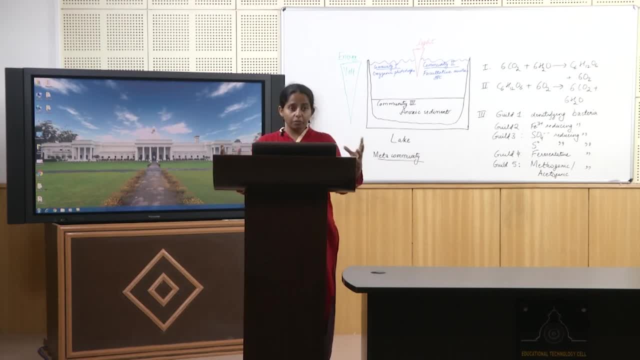 So if there is any glucose molecules floating in the water, it will be trapped in this matrix and then the cells can devour it. So thus we see that biofilms can give a protection to microbes and it can create a nutrient rich environment in otherwise nutrient deficient environment. 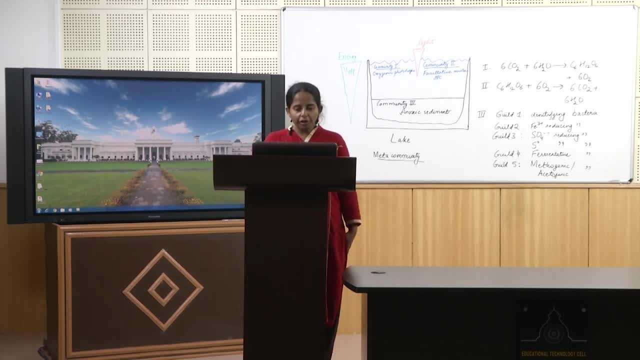 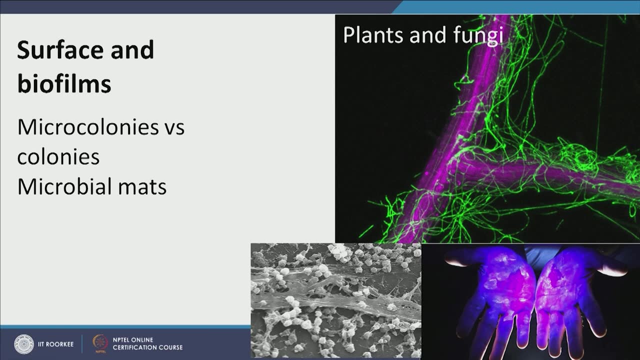 So biofilms are very, very beneficial for microbes. Now. So if you remember, in one of the first few lectures I talked about plating of microbes and culturing. So in plating, what we have is we spread the inoculum over a plate and we spread it in. 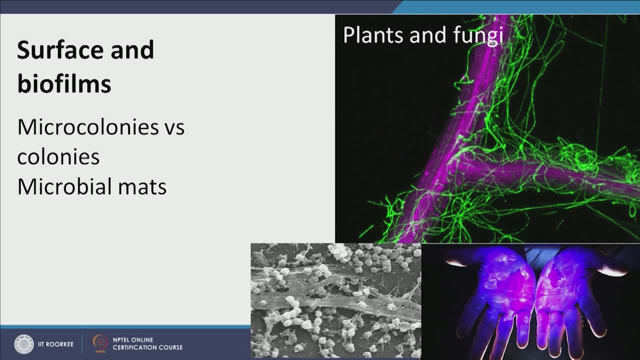 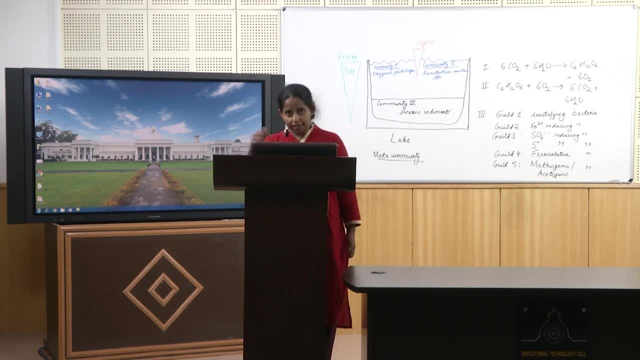 such diluted amount that we expect that when they grow, from a singular microbe, from a singular bacterium, for example, one colony will sprout up which we can see the next day or the day after, after some days. So what the important take home message is that 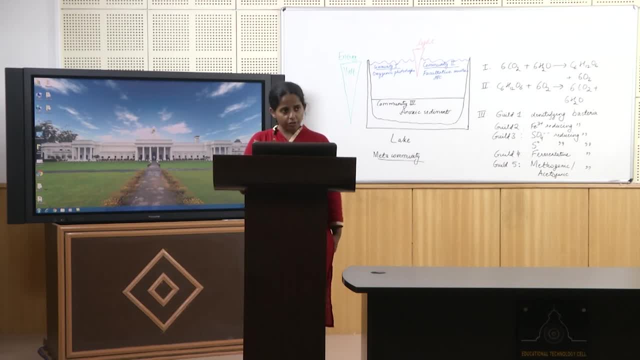 The colony emerged from singular microbes- singular bacteria or some other microbes- and it is visible to eye, So we can actually count them right. However, sometimes in oligotrophic environment, such as very clean streams in drinking water systems, the microbes do not grow into colonies in sense that even though they are source, 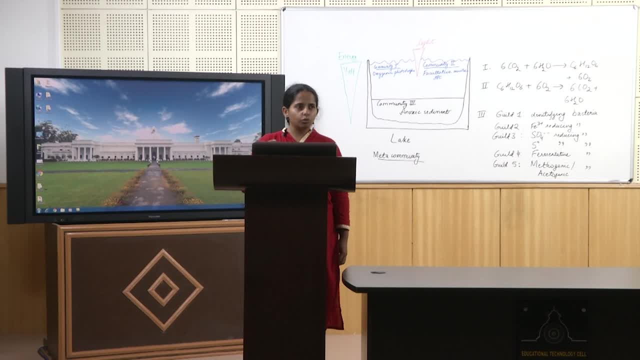 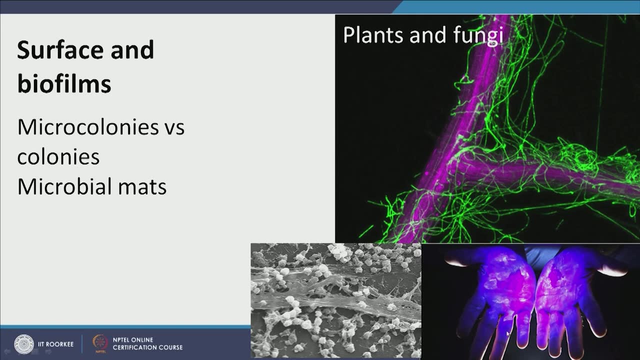 from a single microbe. they make micro colonies, So the only thing is we cannot see them. So, for example, Let us look at this picture on the right panel, right bottom panel. So this is a hand of a person and we are noticing this under dark light. 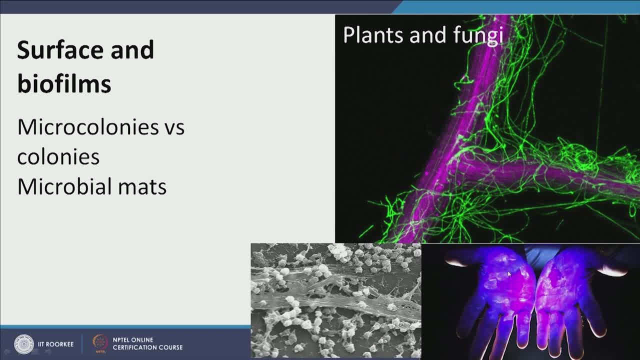 So this is a special technique where we can ask microbes to. we can make microbes to fluoresce, to give fluorescent signal under particular when lit by a particular light. So whatever you are seeing here, giving a fluorescent signal shining, is actually microbial, micro colonies. 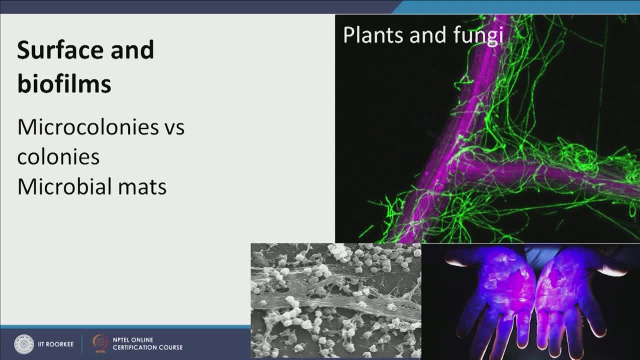 So on a hand like mine, which I believe is pretty clean. So let us look at this picture on the right bottom panel So you can see micro colonies growing and these are the corollary of the corollary particles that are in the corollary. 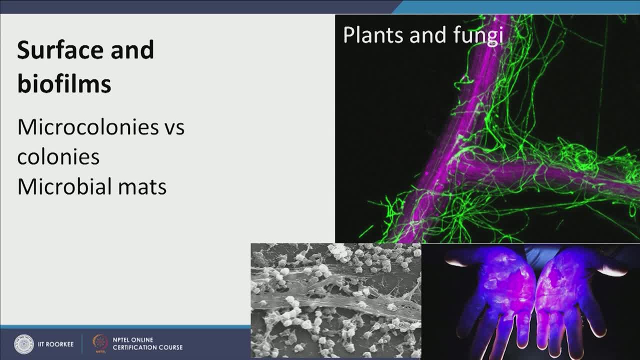 So actually, this corollary is so tiny so that it is pretty noticeable that these are corollaries. Now, if I put my hand between the corollary to the front, this is what is visible. So there are tiny corollaries growing right now. 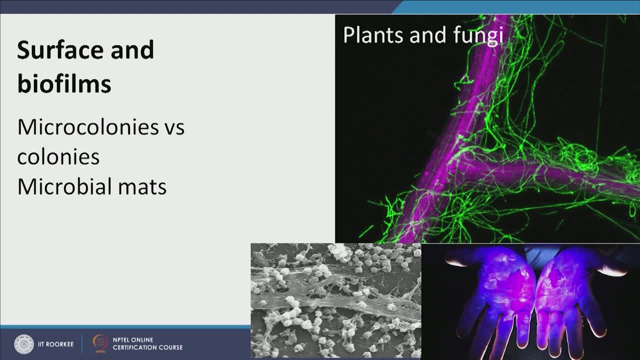 I cannot see micro colonies because they are too tiny, and only when I put my hand under dark light then I can see. oh, there is tiny colonies growing that are otherwise invisible to naked eye, So structurally they are too small to be seen, but the signal can be seen by the eye. 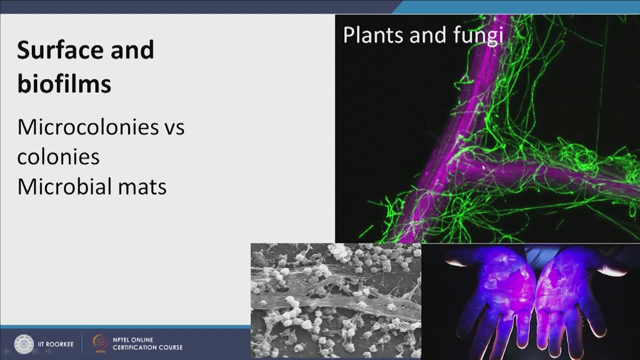 Now, microbes not only make micro colonies in our body, on our body and in our body, but also in other surfaces. For example, in the top right panel we have a plate titled plants and fungi. So in the purple you have root, the root of a plant, and in the green you have fungal. 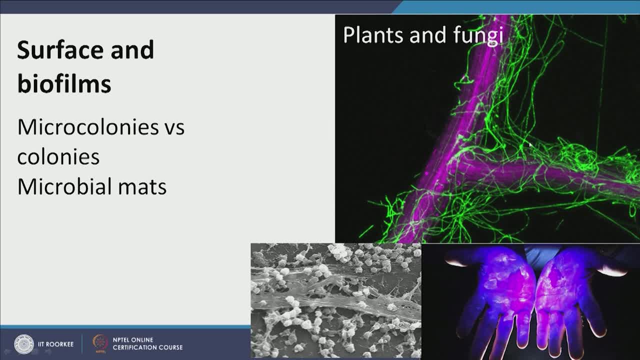 sheath. So the fungus has attached to the root, has entwined with it and is enjoying the nutrient rich environment of the roots and hopefully the root is also benefiting from the fungal attachment to it. So remember it is not just bacteria, but fungus also attaches other microbes also. 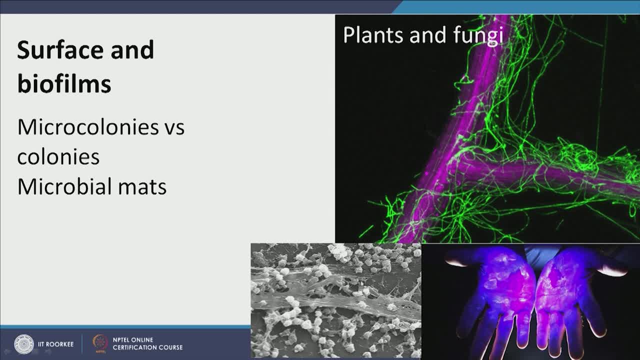 attach To surfaces. here we have another example where we have these microbes who have attached to this surface and this is actually a picture from a microbial mat. So micro colonies are very small. we can see them, colonies. we can see them. both are. 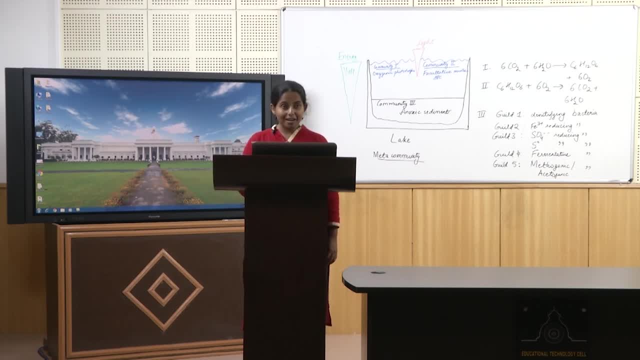 their source is singular microbe. Now, microbial mats are very interesting. they are microbes have populated so much, they have grown so much the biofilms, that they are centimeters thick, and even meter thick maybe, and we can see them. Well, I do not know if meter thick exist. 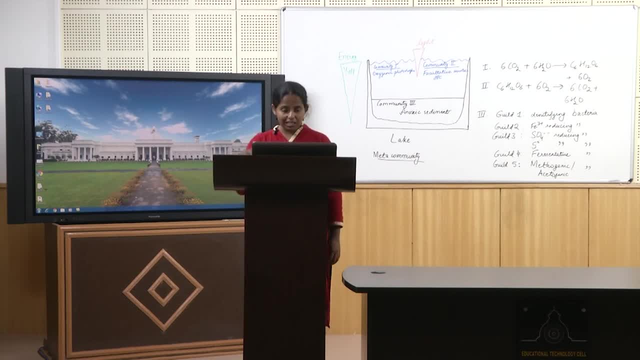 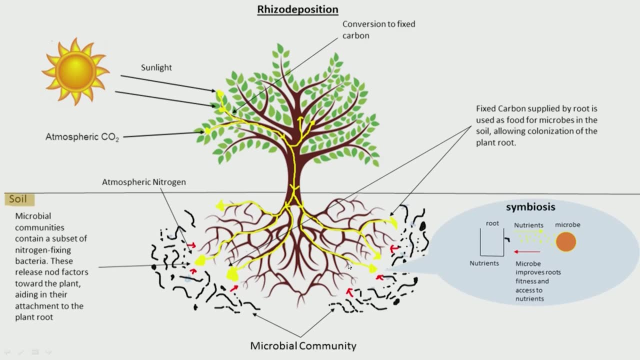 But definitely many centimeter thick. we can see them, we can see the gradation. So let us take a look at that already. before we take a look at that, let us go back to our root microbe interaction. and here we have a plant, a tree, and it is making food from. 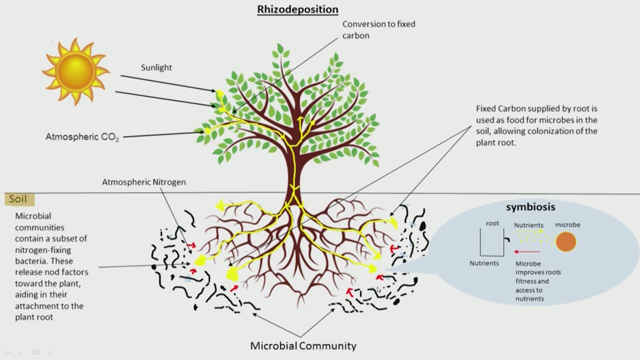 sunlight, carbon dioxide, water and in its root it is using roots to get water and other resources that it requires, and you will notice that the roots provide a fixed supply of carbon, the yellow line, The yellow line or nutrients, to these microbes here and these microbes in other. on the other, 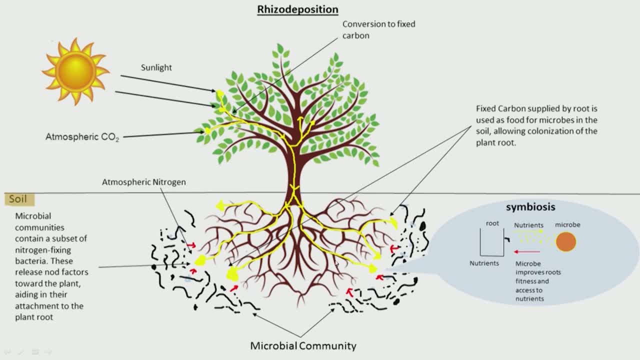 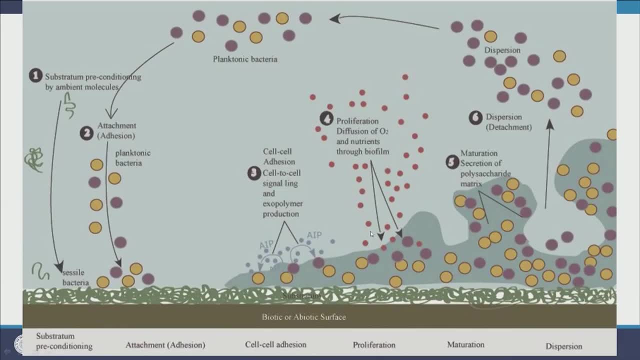 hand fix the nitrogen and they provide nitrogen source to tree. So this is a very good example of symbiosis, alrighty. So now let us take a look at microbial growth on surfaces. So the first one we have here: we want to understand how biofilms grow and how microbes 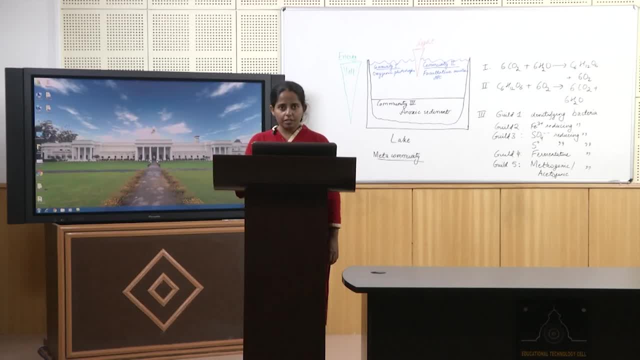 proliferate in them. Later on, when we will be talking about drinking water system and drinking water treatment, it is very important, So it is very important, to understand how biofilms will grow in our drinking water system, and this is a big challenge, by the way. 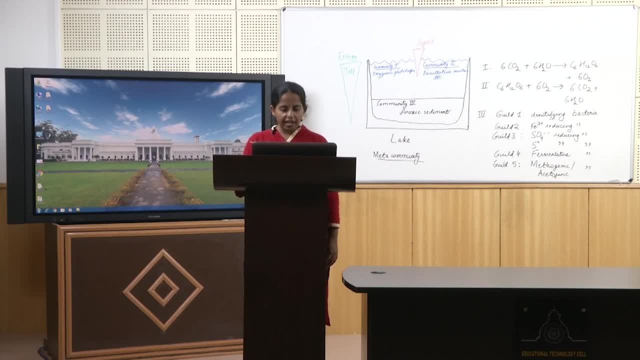 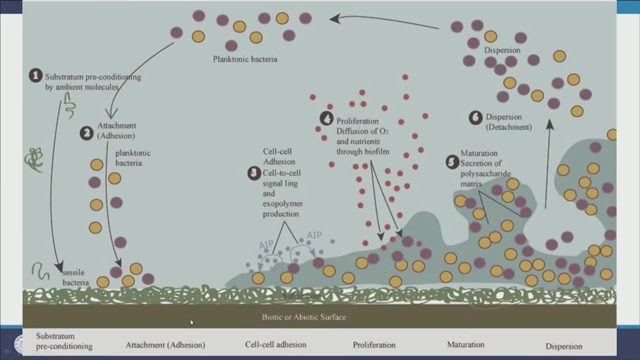 So let us get our fundamentals right here. So in this picture we have six different stages of biofilm formation. The first stage is substratum preconditioning. So initially this is our biotic or abiotic surface. So biotic surface would be like root or like a teeth or like my hand or hand. abiotic could 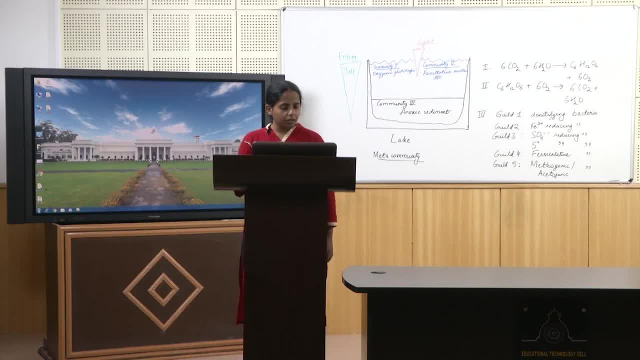 be like a pipe material or a wall right Now, or like a catheter. Then we are talking about medical devices. So we have these sessile bacteria. they will go, they will attach to the surface and they will prepare the surface for better attachment by live microbes. 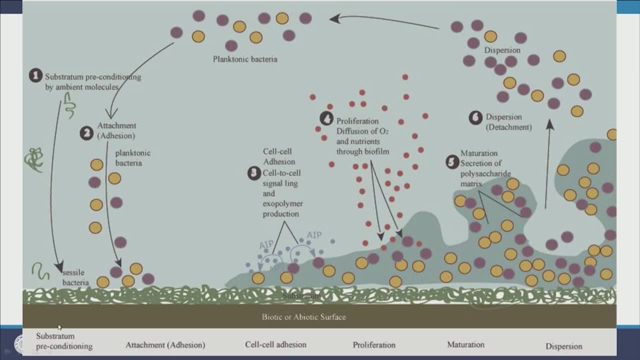 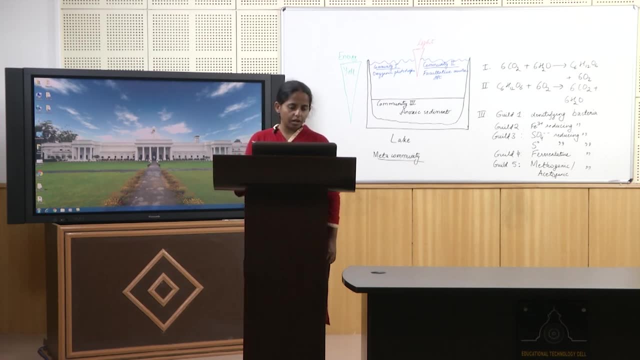 So the sessile bacteria have attached and they have conditioned the substratum. The substratum is now ready to be sticky to allow things to stick to it, And now we have these microbes in yellow and purple color. they are planktonic bacteria. 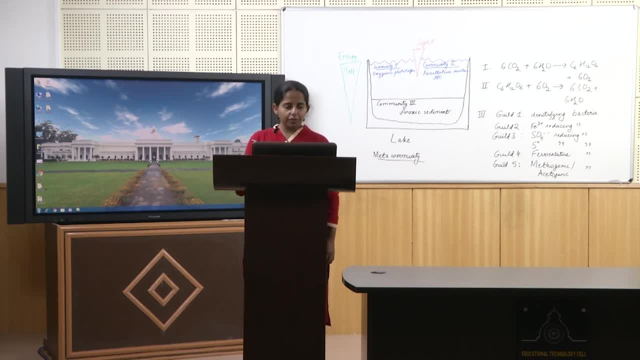 what means? they are free, freely floating bacteria. So here we are imagining this blue environment, So we have this blue environment, So we are imagining this blue environment to be water, So they are freely flowing bacteria and they are coming, and now the surface is ready for. 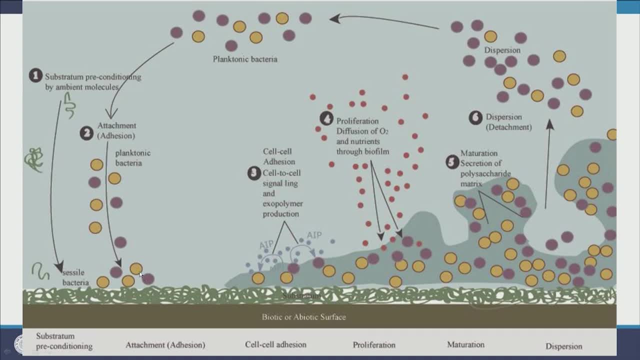 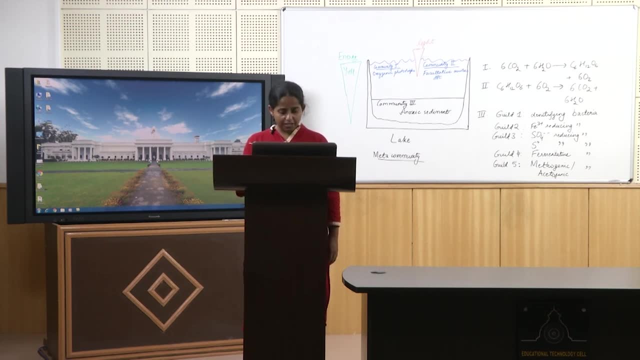 attachment and then they get attached. When they get attached, not only do they get attached to the cell surface, but they also get attached to each other. So what we notice in the third step is cell to cell adhesion. So these microbes, they start talking to each other using chemicals. 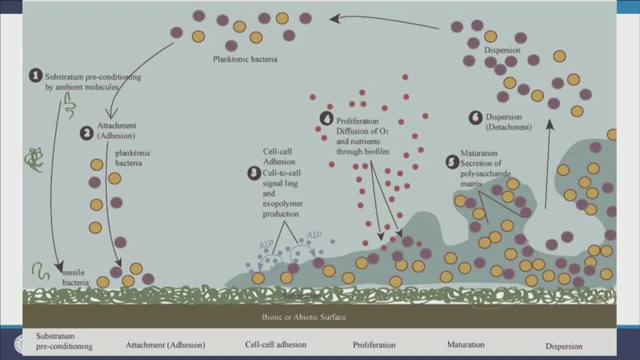 So they do biosignaling, cell to cell signaling, and they tell: I am here, who else is here, how many of us are here? Are the other microbes present here? are they enemies, are they friends? are they going to compete, are they going to cooperate, are they going to have predation? 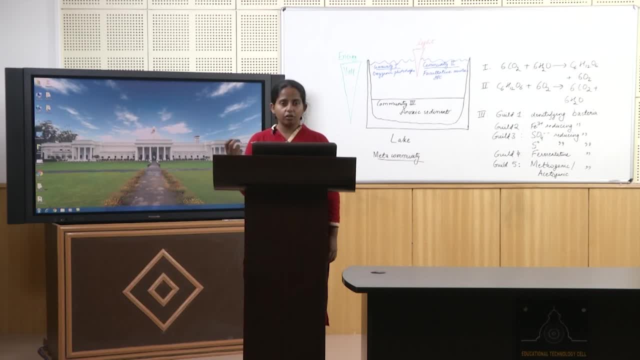 So they communicate with each other and then they stick to each other according to whatever serves them the best. So they stick to the ones when sticking is beneficial. So they have cell to cell adhesion, cell to surface adhesion and they have a very nice. 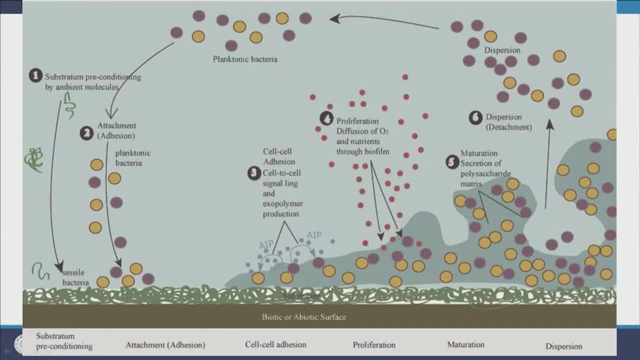 communication network. Now, at this stage, they also start producing the exopolymer. So this is EPS which they produce. so this is a net that they cast. So if you see here dark blue, darker shade of blue here, this background environment, 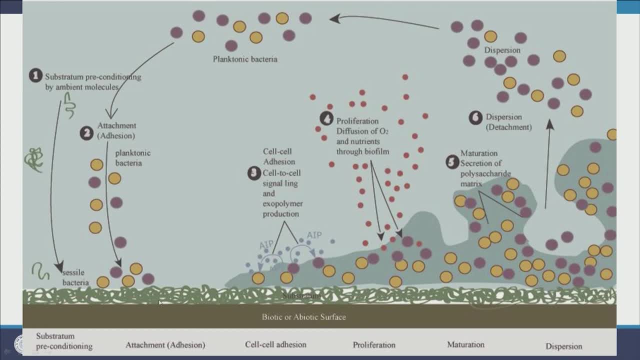 is the EPS that they have made. So initially there was no EPS, just the surface was ready to exit microbe. but now we have EPS layer that will trap both nutrients and trap the microbes. Now in the next stage we have proliferation. 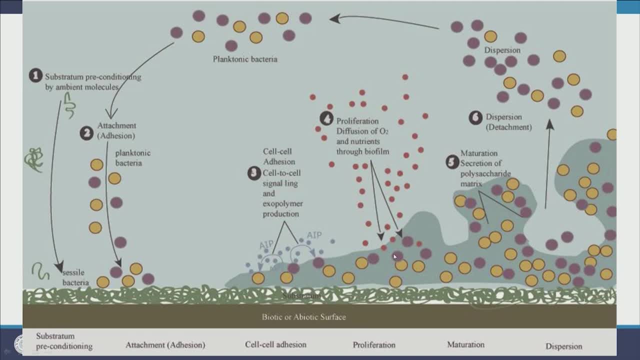 So in proliferation, this biofilm that has grown and this EPS structure that has grown here, So this biofilm, microbes and lot of EPS structure, they will start trapping food. so nutrient, so diffusion of oxygen and nutrient through biofilm. because this is a pipe, got schematic. 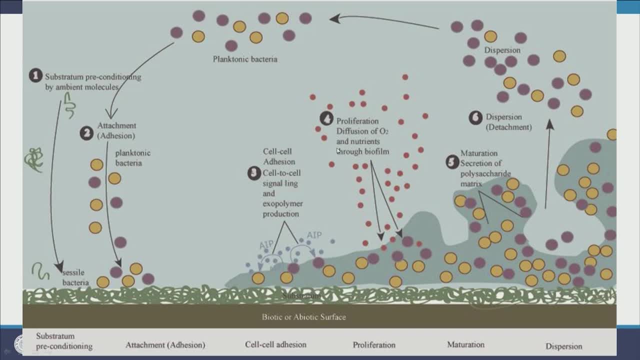 showing how biofilms grow in pipes. so we are talking about oxygen, but it does not have to be necessarily oxygen, as we will see later. But the nutrients- electron acceptor, electron donor and everything else that is required- will start diffusing into these biofilms and the microbes will start proliferating, which 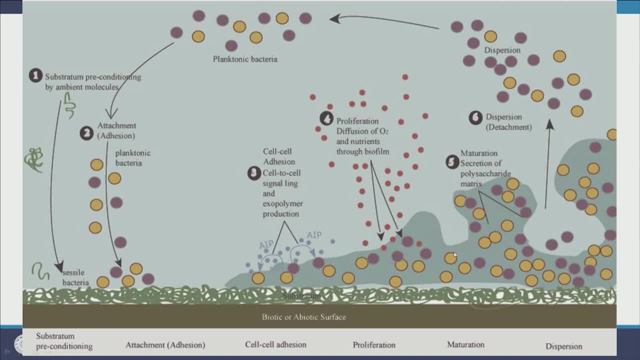 means they will start growing in population And then they will start producing biofilms. So they will start producing biofilms And then, when they start growing in population, they produce more and more EPS and they make more complicated structures, and this is maturation. 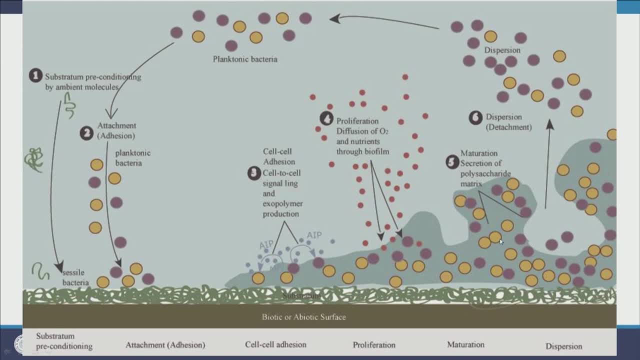 So they are now secreting polysaccharide matrix, EPS, and now they are having more complex structures and very diverse microbial community by normally by this time. Now note here: they allow diffusion of oxygen and nutrients. let us say we have a disinfectant. 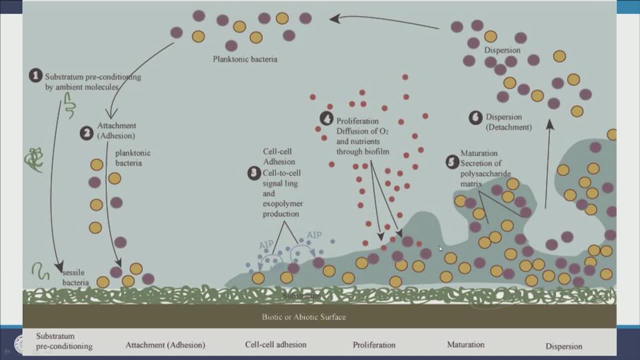 in the environment. Now this disinfectant will also diffuse but will only affect microbes who are at the boundary. And some microbes here will survive, and once the microbial community in the biofilm becomes more and the biofilm becomes more mature, then the population of surviving microbes 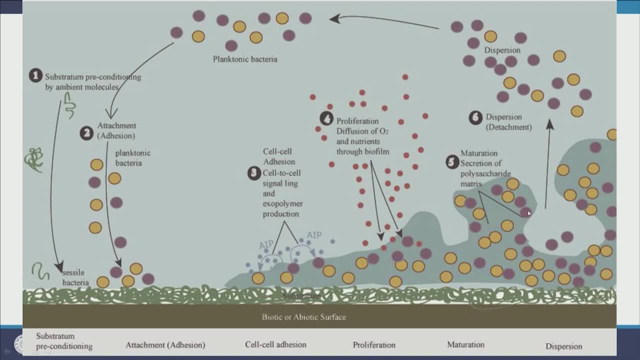 in phase of disinfectant would be much higher than microbes that do not survive. After a while, when the biofilm grows too much that it is structurally unstable and the microbes are too populated, they are ready to find new avenues for attaching and for. 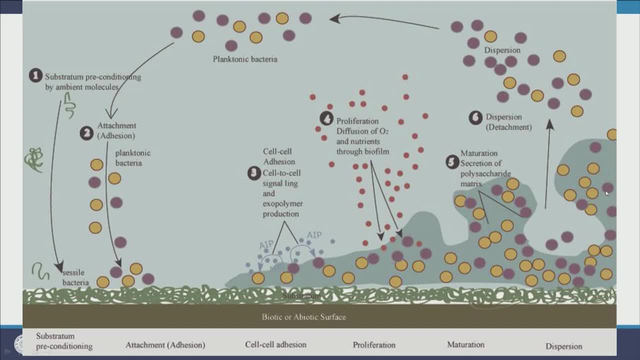 growing, then they will have dispersion. So this is where the biofilm releases itself breaks out open. So this is where the biofilm releases itself breaks out open. So this is where the biofilm releases itself breaks out open. 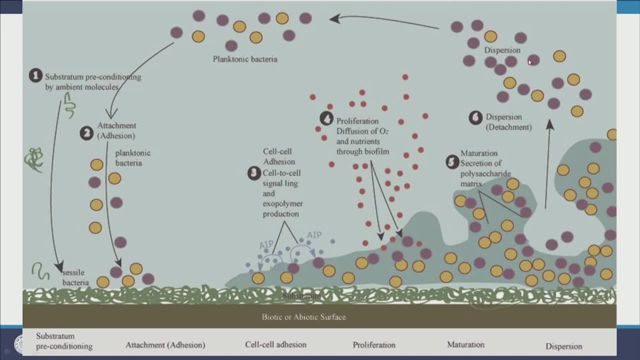 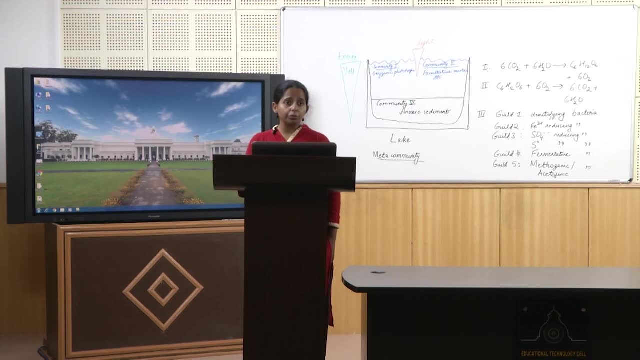 And the microbes are released back and they become planktonic bacteria. And the microbes are released back and they become planktonic bacteria. Now this is where the problem is. Let us say there was a pathogen hiding and proliferating here. Some pathogens can proliferate in biofilms. many cannot, but some can. Or let us say, just someone was surviving here, saving itself from the disinfectant and getting the minimum nutrients it requires to survive in such an oligotrophic environment. Now, in this stage, when they are released back into the water, then this water can be drunk. 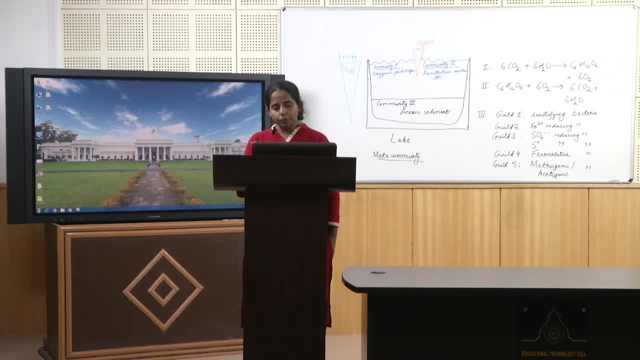 by a human being or by some other being. So when we open the tap and we get this planktonic bacteria, some of them could be pathogenic and next thing we know we are falling sick. The other fate of planktonic bacteria is that nobody drinks them, but they find more attachment. 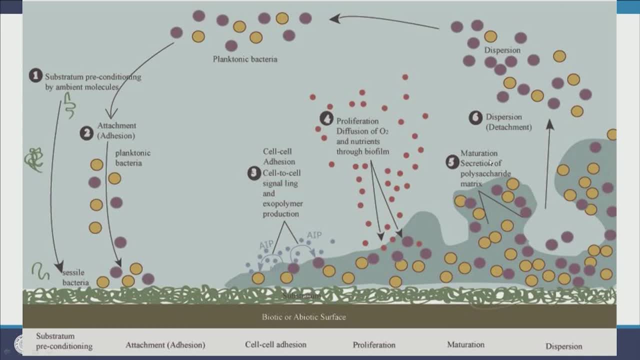 surface and they attach. So you can see this is a cycle and they induce each other. So more biofilms produce more biofilms. one begets the other. And next thing, we know that our drinking water system is afflicted with a certain amount of 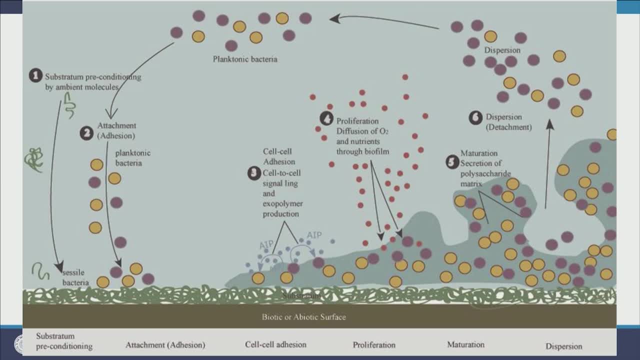 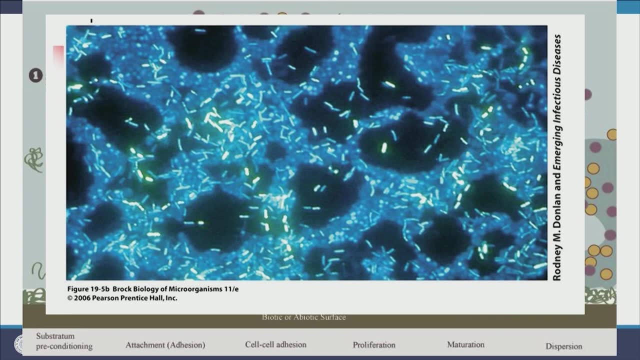 biofilms. So biofilms are rampant in our water distribution system. Now this is a picture you might think. how will microbes attach to something like a metal surface? This is a picture showing microbial attachment to stainless steel surface. So we have stainless steel surface in the background and all these fluorescence that 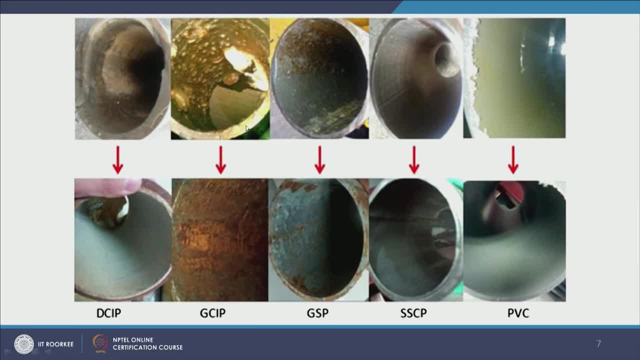 you see here is from microbes, All right, and this is a picture of different pipe materials. So in the right we have PVC, here we have different kinds of metallic pipes and we notice how biofilms develop, How they aid in corrosion. We won't get into depth here, but later on, when we talk about drinking water treatment. 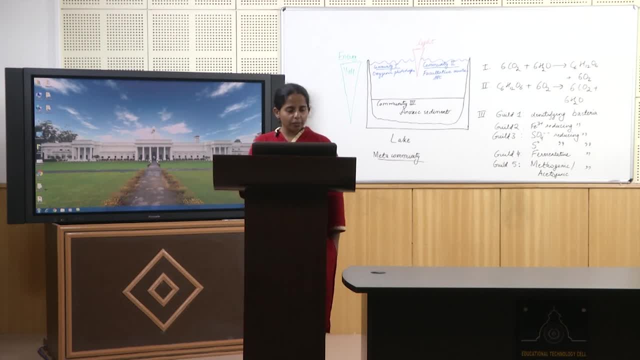 I'll talk more about this. The other example of biofilms would be our teeth. So remember, this is not just all plaque that forms in our teeth, but now we have biofilms shining in our teeth. Now let's talk about microbial mats. 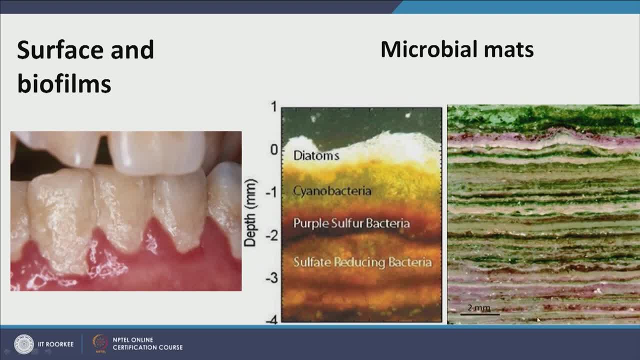 So, as I said, microbial mats can be multiple centimeters. So here we have nearly 2 centimeter long deep microbial mat. So we have different layers. So, as I said, microbial mats can be multiple centimeters. So here we have 4 millimeter depth of microbial mat. 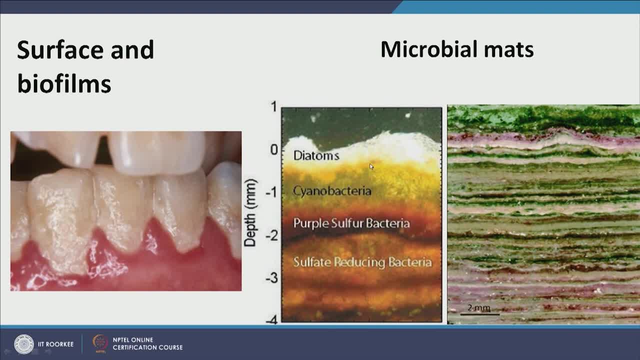 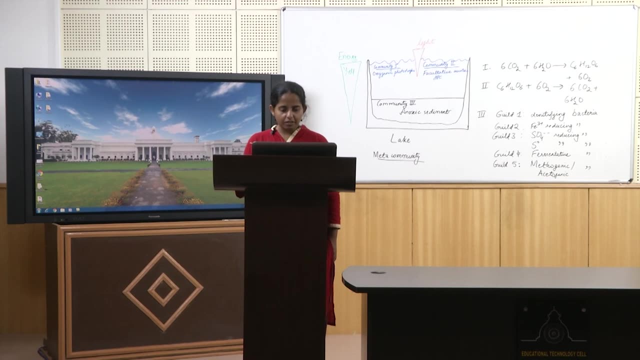 Let's look on the top we have diatoms, Then we have their special kind of algae, who are very highly sophisticated and, I might say, microscopically very beautiful cell wall kind of structure. And then we have cyanobacteria, and we have purple sulfur bacteria and we have sulfate. 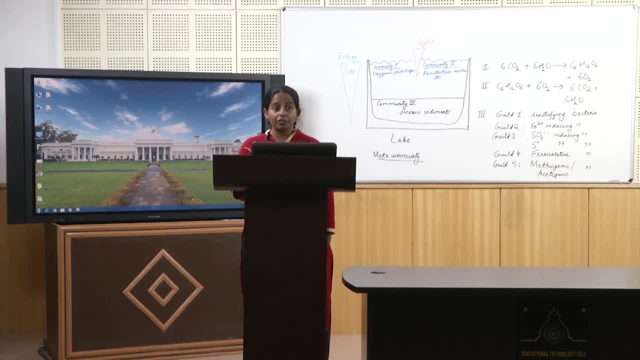 reducing bacteria. So you can see, not only do we have layers of microbes, but we also have layer of functions. and if you remember, what is a guild? a guild is microbes of similar functional nature. so this, these are guilds, these are layer of guilds. so if 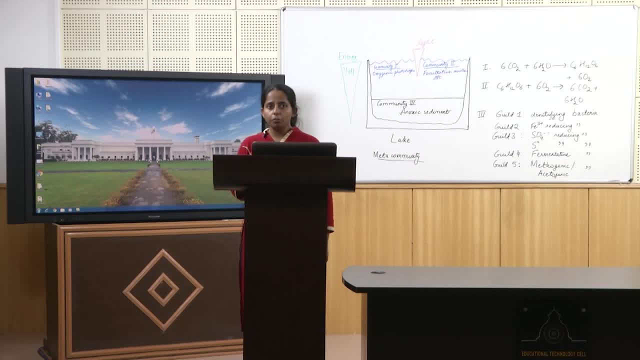 we are reducing bacteria. you know they can be different, they can belong to different phylum, so they can be very different, but they are all same function. so this is a guild. now let's look at some very exciting microbial mat usually found in the coastal regions of 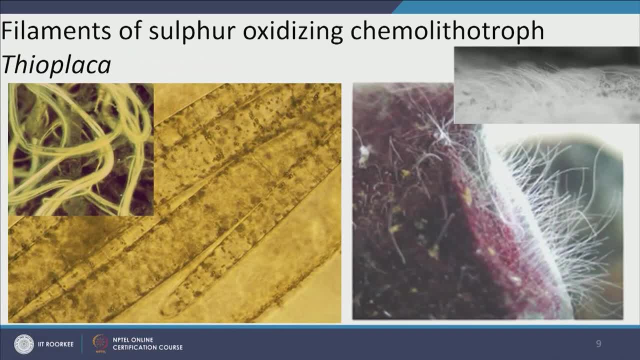 chile and peru in south america, and this is a sulfur oxidizing chemo, chemolithotroph, thioplaca. now, thioplaca oxidizes sulfur and it's a chemolithotroph and it forms filamentous microbial mat that can go up to 5 to 10 centimeter below the sediment. so we are not just talking. 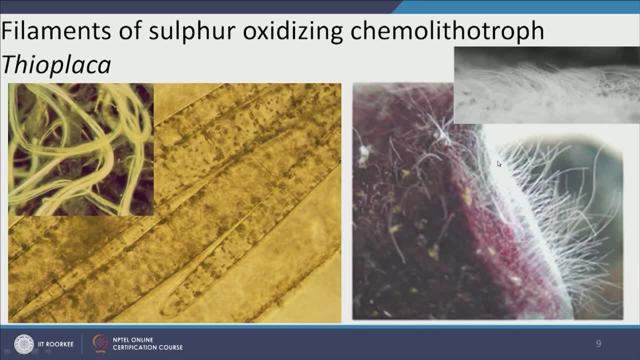 about 2 centimeter here, as we were talking about the sediment. but we are talking about 2 centimeter here, as we were talking about the sediment. so we are not just talking about here, but here we are talking 5 to 10 centimeter below the sediment, and then they have these. 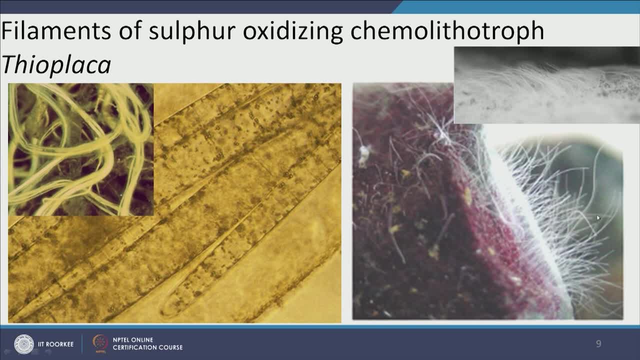 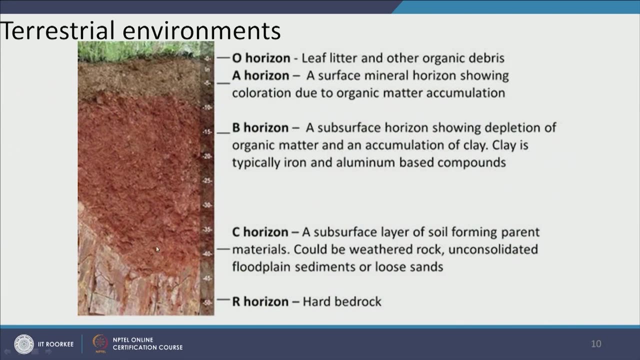 hair like filaments that they have outside. these are sheets that actually allow that whole thioplaca together. so this is a microscopic picture. another and these are other beautiful pictures from chile and peru. now let's look at terrestrial environment, as promised. now this is a well mature soil, so not just uh, okay, why would microbes form a gradient? 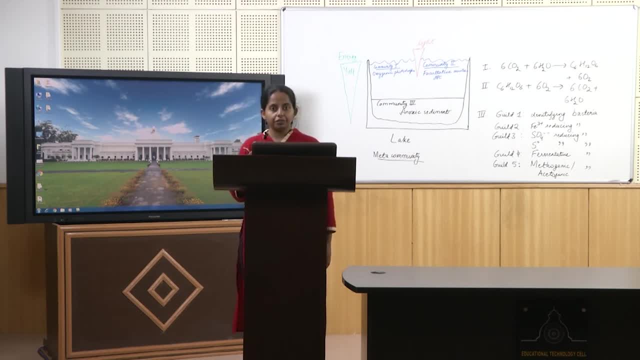 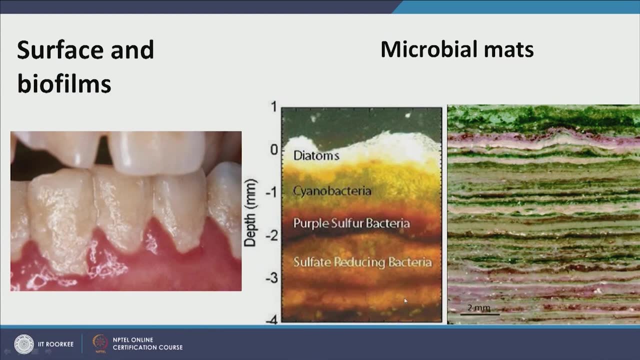 why will they go from diatom to all the way to sulfate, reducing bacteria, as we saw in this microbial mat? because the environment is changing. this is oxygen rich and then oxygen gets depleted. as oxygen gets more and more depleted and let's say, for some reason the reaeration is stopped. 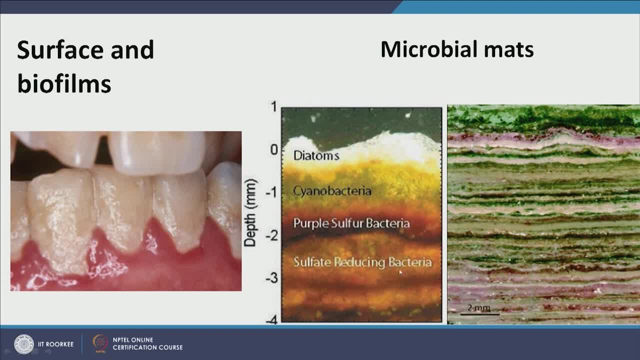 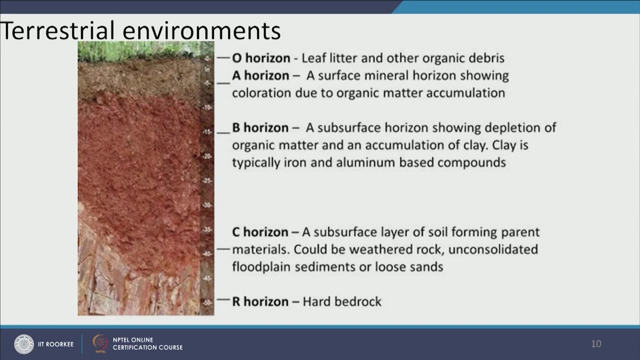 then the sulfate reducing bacteria will occupy more volume than the other, and when sulfate is gone, then we'll have fermentation or another electron acceptor being reduced. okay, so, and you know, it's not just microbes that form gradient, but in nature too, we notice that the environment is. 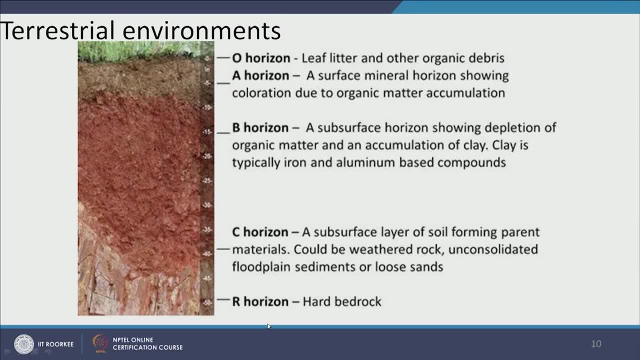 has a gradient. so this is a fully mature soil and at the bottom we have our zone, our horizon, which is a hard bedrock. then we have c horizon, which is a subsurface layer of soil forming parent material. this could be weathered parent material for the soil. this could be weathered rock. 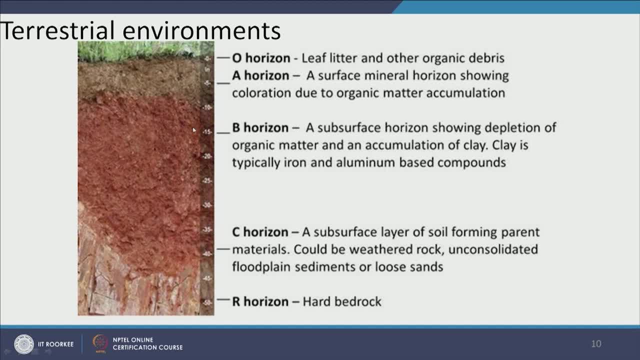 unconsolidated floodplain sediment or just loose sand. then we have the b horizon here, which is a subsurface horizon which is showing depletion of organic matter. so we have rich organic matter- dark. so rich organic matter gives soil dark color, but here the color has been lost. so we have a lot of clay and we have depleted organic matter. in a we have 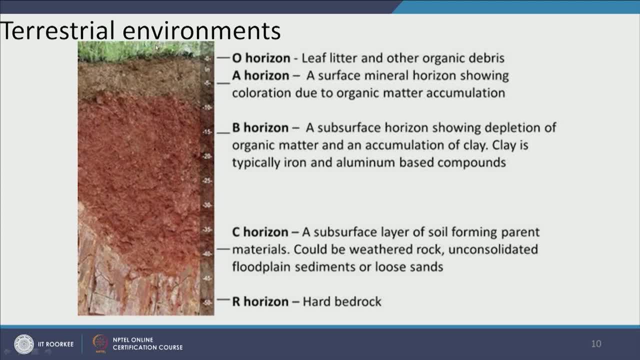 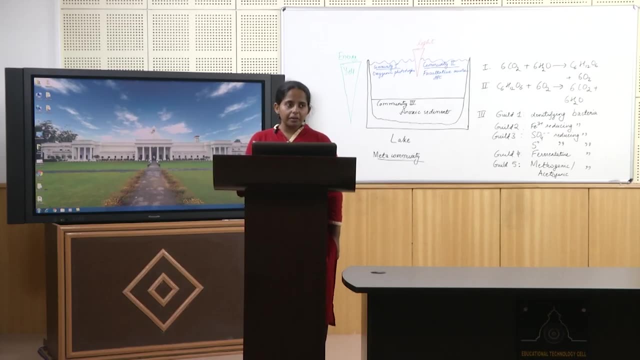 dark coloration because organic matter has accumulated in the? o. we have leaf litter, so we have a lot of biomass waiting to degrade and waiting to make the soil darker in color and make it rich. as i talked earlier about micro environments, terrestrial environments are very complex for many reasons because- think of it this way- each pore in the soil and even in a small 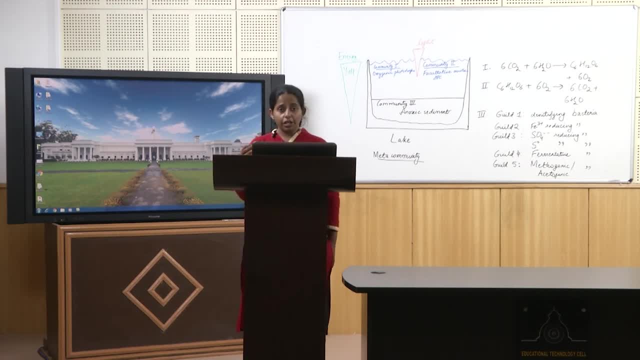 handful or spoonful of soil, you'll have so many pores. each pore is a micro environment and within this micro environment we have gradient of nutrients, we have gradient of electron acceptors and even we have some pockets within micro environment that will have water, some will not. 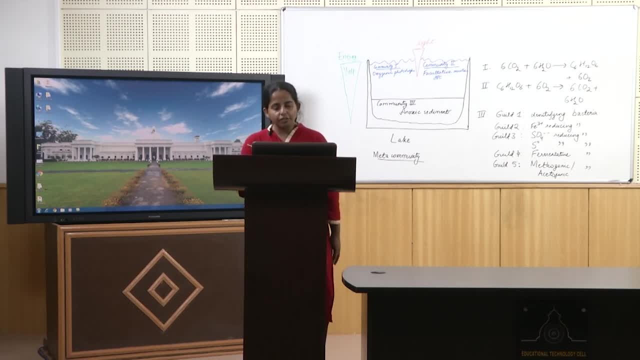 have water, as illustrated by this schematic. thus we can expect very diverse microbial communities in each pole, and you know, pores adjacent to each other might have very different microbial communities flourishing. one might be anaerobic, the other might be water loving aerobic. so let's look at this little micro. 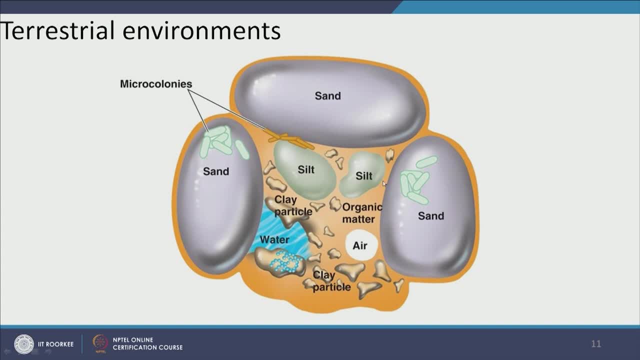 pore. we have sand particles, we have some silt, we have some clay, small clay particles. it has air trapped, so oxygen in this air would be utilized until there's no oxygen left and then, because there might be nitrogen and other things, we might have nitrogen fixing bacteria or other kind of microbes. now, in each of these zones we have 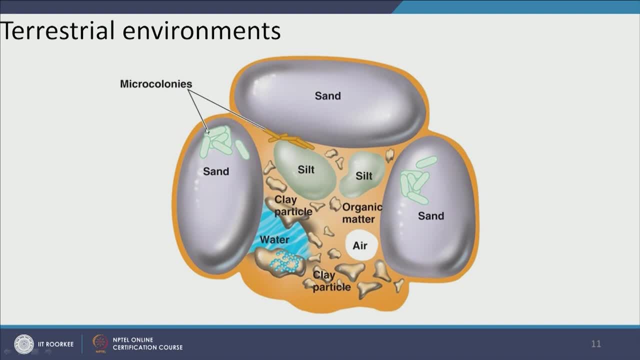 micro niches that are perfect for a particular kind of microbe to grow. so microbes that love binding to sand will probably stick to sand and grow there. the ones that love to grow between silt and sand or stick on silt will grow sticking on silt. the ones that love to grow in water will. 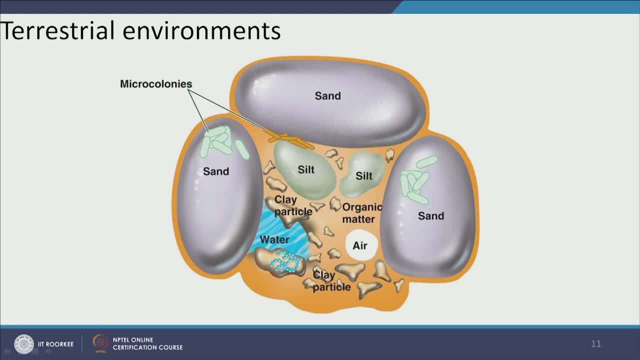 grow wherever they find little trace amount of water within the micro pool, and we are talking really small environment here. yeah, so we notice that there are a lot of nutrient diversity and even as air gets extremely consumed here, initially we'll have aerobic microbes here. then, when air gets, 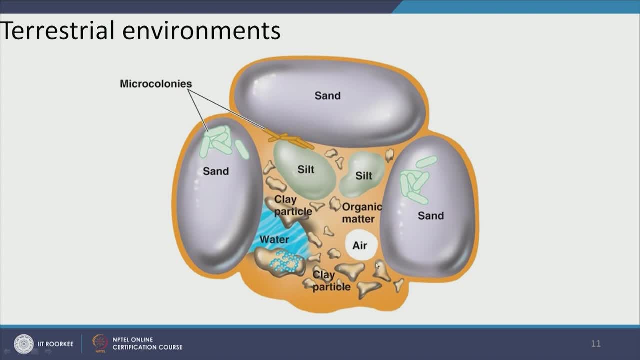 oxygen gets consumed it will move on to um, non-oxygen electron acceptor zones, such as microbes that use nitrate, microbes that reduce sulfate or sulfur, and eventually to methanogen and fermentation, fermentation and methanogenesis. so we will see both electron acceptor gradient. we will see nutrient gradient and water gradient. some. 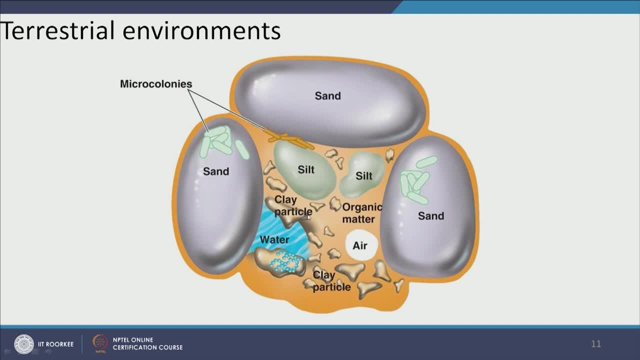 love water. some like to like water, but they like to keep the distance, so they will grow in this region instead of growing in this region. now, um, for example, here i showed you microbes that love to stick to sand. now there are microbes that, um, what they do is- and this is a electron, um. 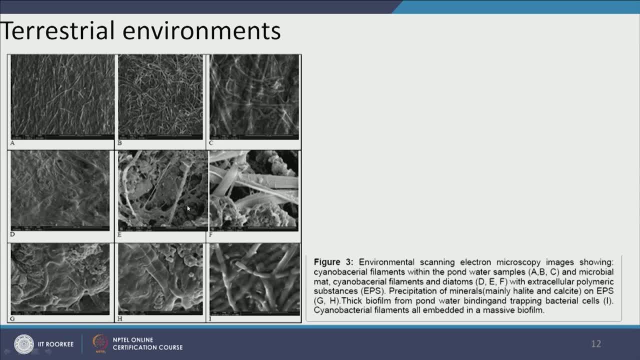 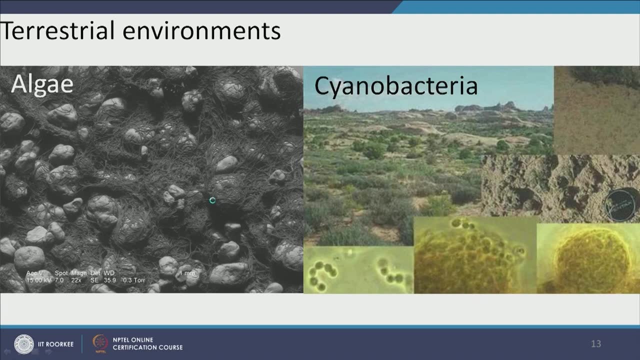 scanning. this is scanning electron microscopy image that is showing you cyanobacteria, by the way, and these are filaments and what they are doing is um. in this they the filaments and the sand traps the microbes. so the sand is what is trapping the microbial, like how this picture shows you. 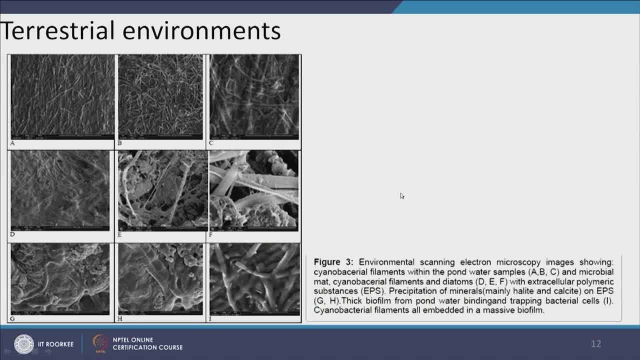 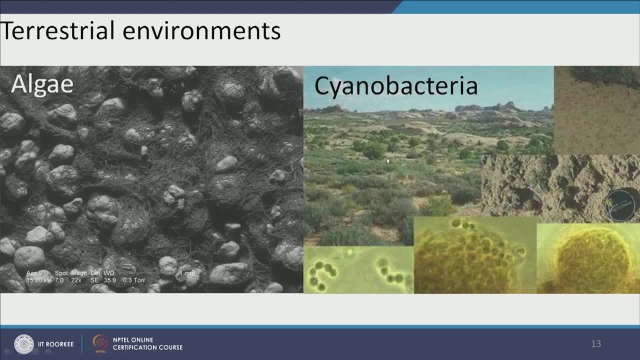 the sand is what is asking: microbes come and stick to me. so this is what this picture is showing, but here we have a very different phenomena happening. we have loose sand particles in desert and in this particular example, we have cyanobacteria, again like here, and here we have 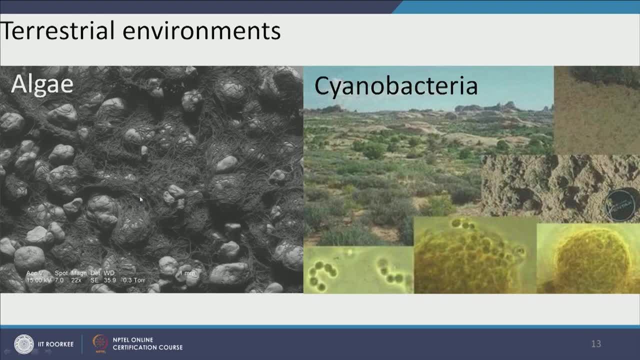 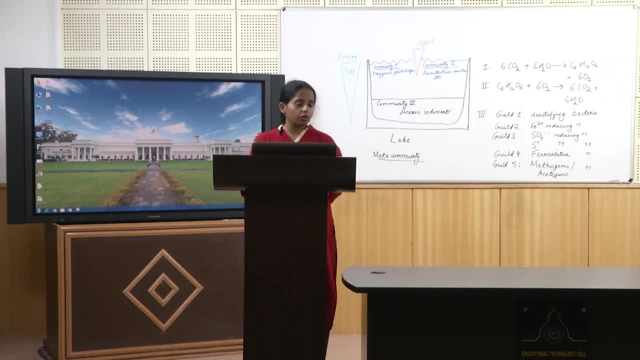 algae and they are binding the soil, so both the microbes can be trapped by the soil, can be trapped by the sand, and then they will proliferate there, grow there or undergo succession, or they can actually change their environment by binding the. so here all these sand particles are very 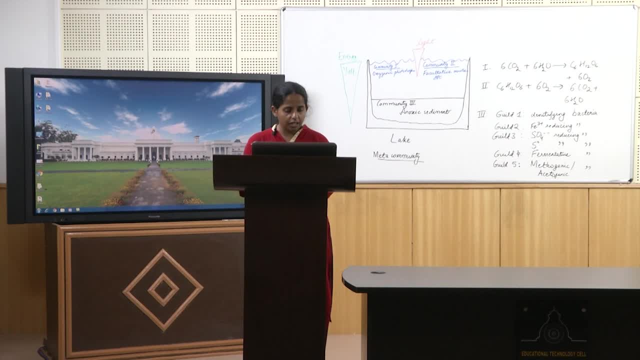 they're not attached to each other. they can disperse very easily, but the algae has grown in and around them and bound them together. so next thing we know the soil is very compact. it's not loose. you won't have sand blowing on your face and similarly, here's the desert in. 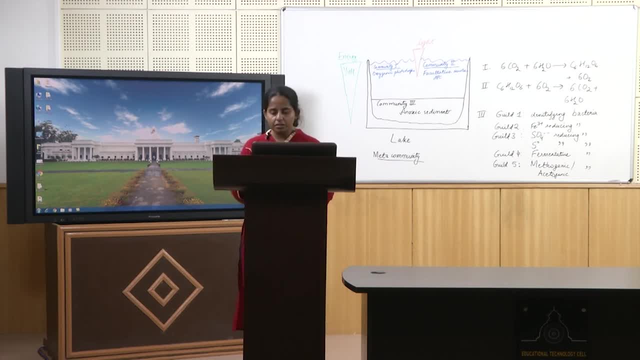 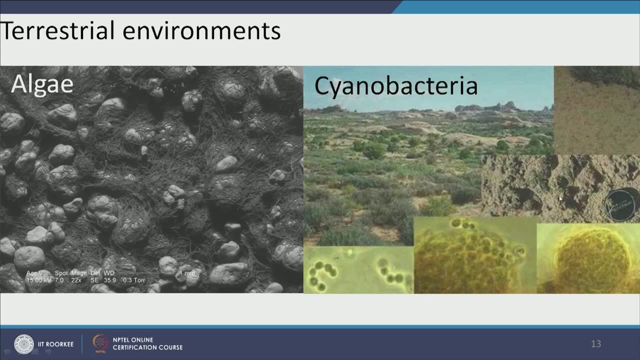 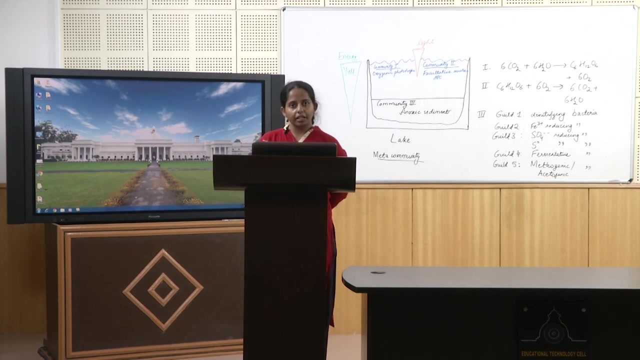 usa, where they conducted investigations, intensive, comprehensive investigations, and they found that it was cyanobacteria that was actually binding the sand particles together and thus changing the characteristics of soil and changing the characteristic of vegetation now within soil. as you now notice that there are different micro environments, there are different. 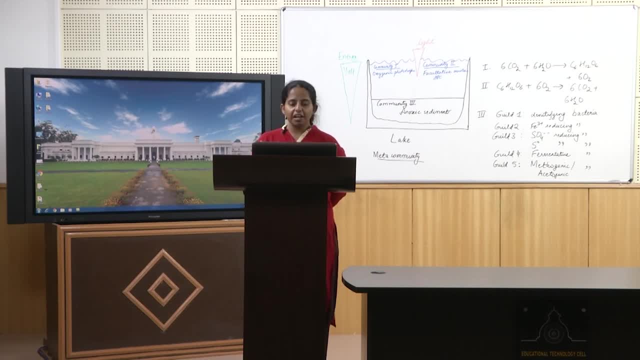 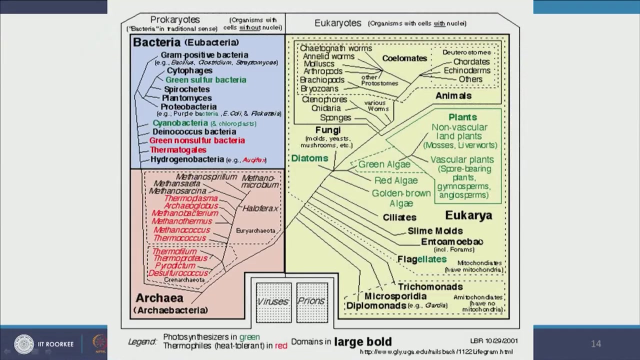 functional gills, and thus we notice a very, very diverse microbial communities in our soil, and this is just a snapshot of some very basic eukaryotes, archaea and bacteria that have been known to find in the desert and soil. each of these kingdoms, whether we go to, eukaryotes or bacteria or archaea, 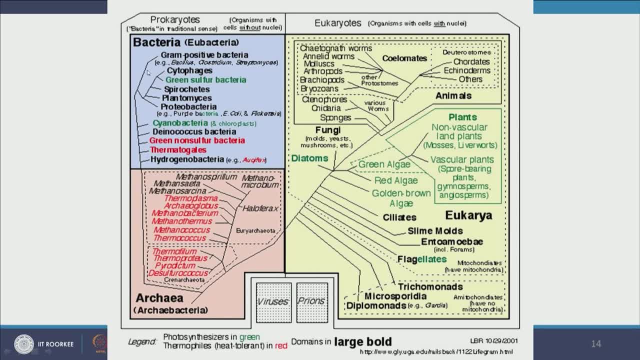 each of them are very, very diverse, so we can't say that, oh soil. you'll have gram-positive bacteria, spirochetes, plantomyces, myces or proteobacteria. you'll have a lot of microbes and within each of them, for example, proteobacteria is a very, very broad phylum. within proteobacteria, we have alpha. 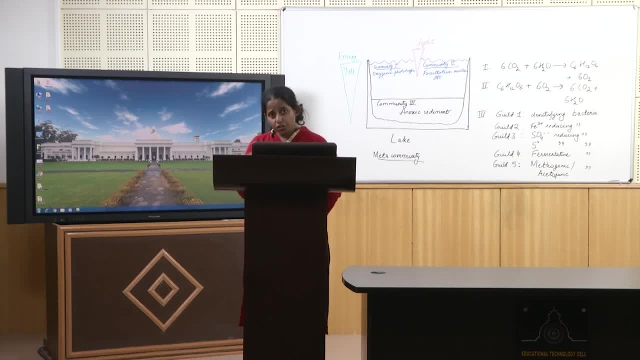 beta, gamma, delta and epsilon proteobacteria, and within each of them we have very different kinds of microbes. for example, some delta by delta proteobacteria are sulfate reducers, some are sulfur oxidizers. some are aerobic and they don't care about sulfate reduction or sulfur oxidation. 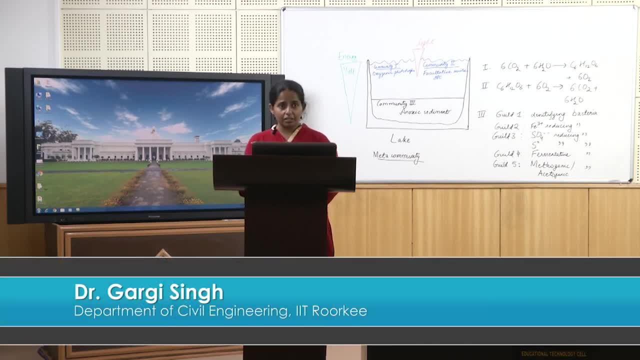 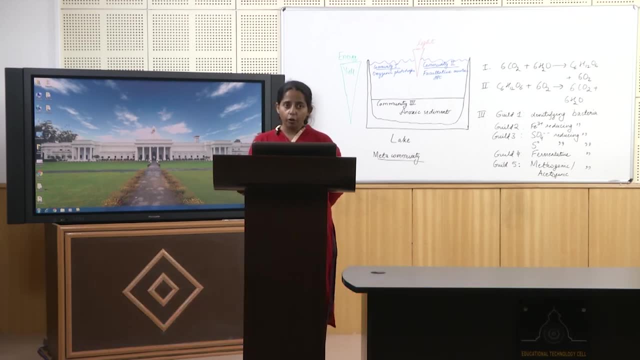 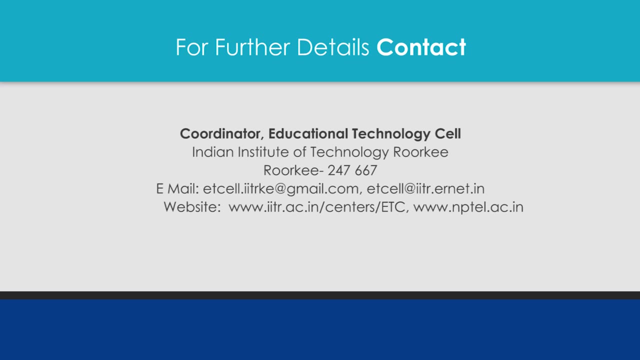 so, as you notice, microbial communities and soil interest terra are very, very diverse. so, my dear students, this is all for today. in next class, we will move on to aquatic environments and we'll see the ecology of aquatic environments. thank you you. 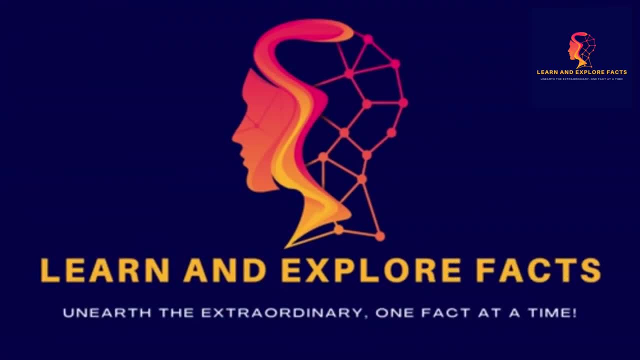 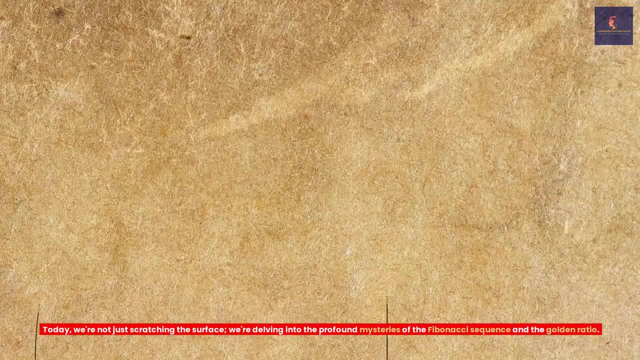 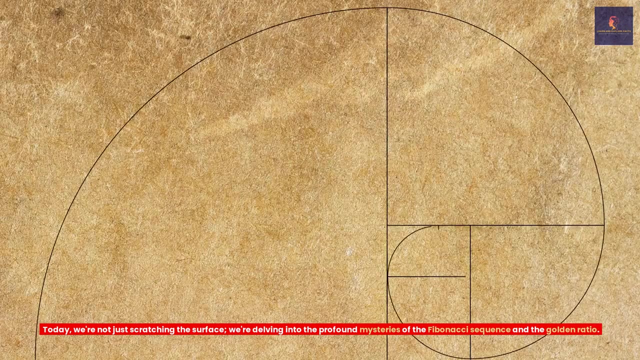 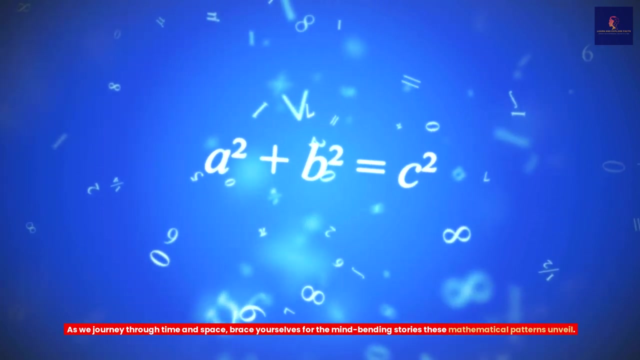 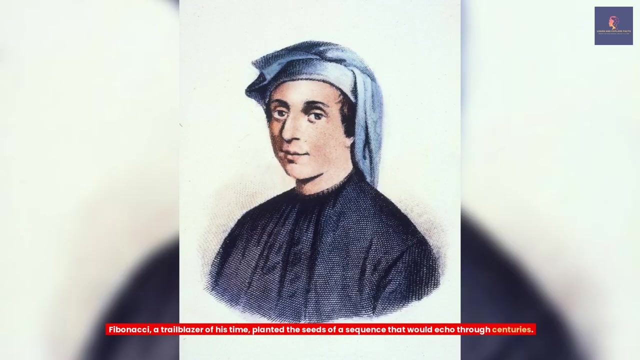 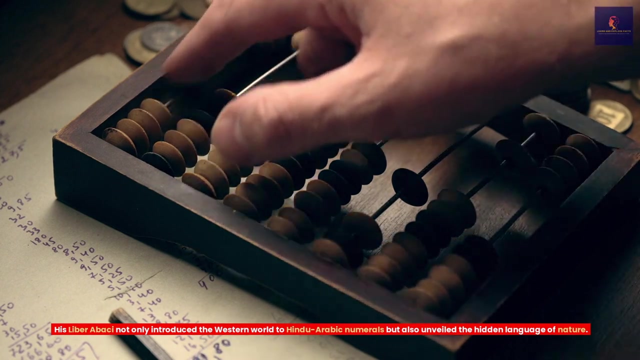 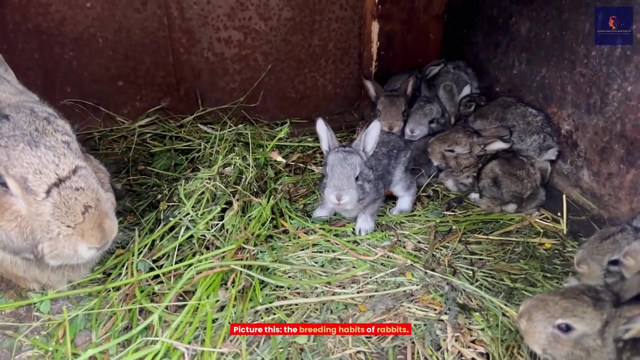 Thank you for watching. A trailblazer of his time planted the seeds of a sequence that would echo through centuries. His Liber Abaci not only introduced the Western world to Hindu-Arabic numerals, but also unveiled the hidden language of nature. Picture this: the breeding habits of rabbits. 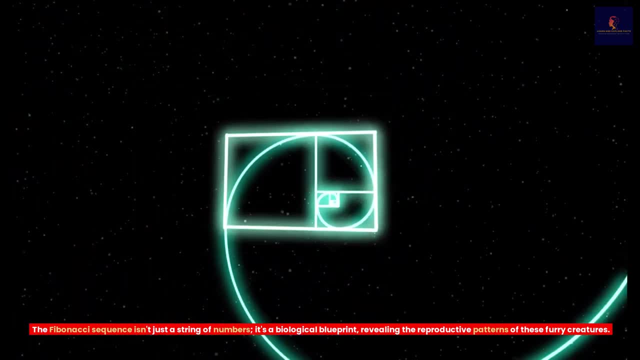 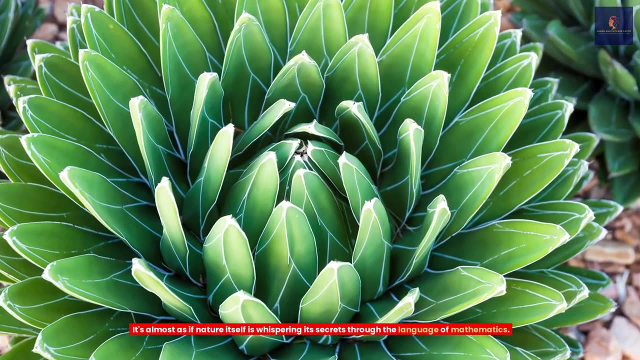 The Fibonacci sequence isn't just a string of numbers. it's a biological blueprint revealing the reproductive patterns of these furry creatures. It's almost as if nature itself is whispering its secrets through the language of mathematics. Now let's venture into the heart of nature's.